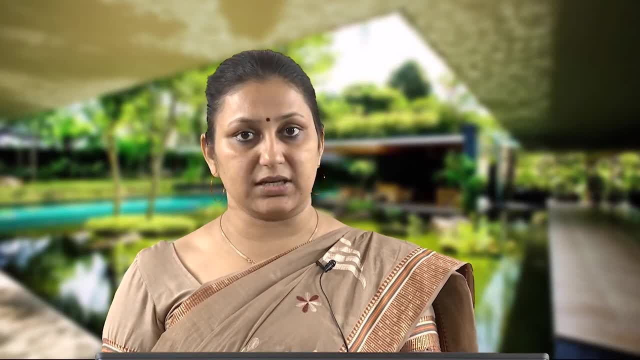 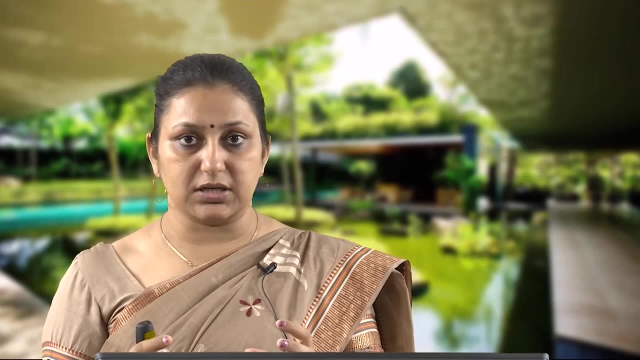 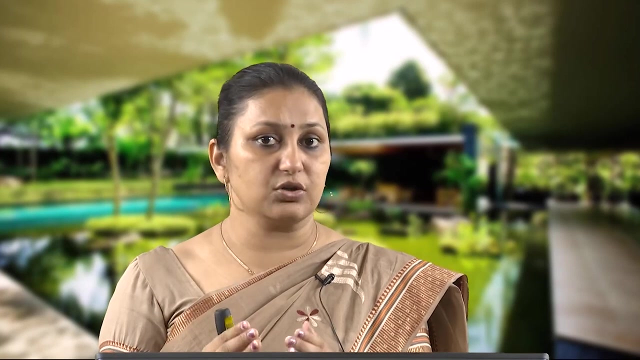 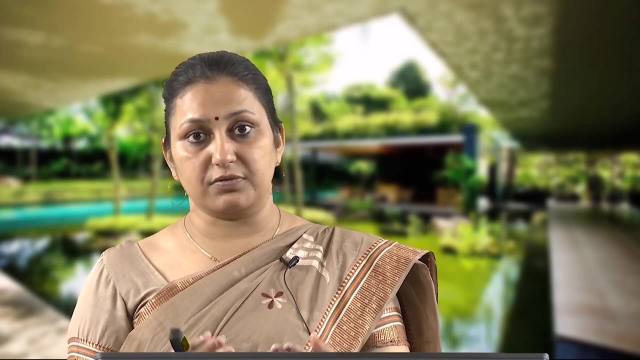 the visual and acoustic comfort which also needs to be taken care when we are designing buildings. and since we started talking about the sustainability in buildings, we have discussed that human beings, the occupants, the users- are at the center of these buildings, and these buildings have to be designed for the human beings, keeping in mind the comfort of these. 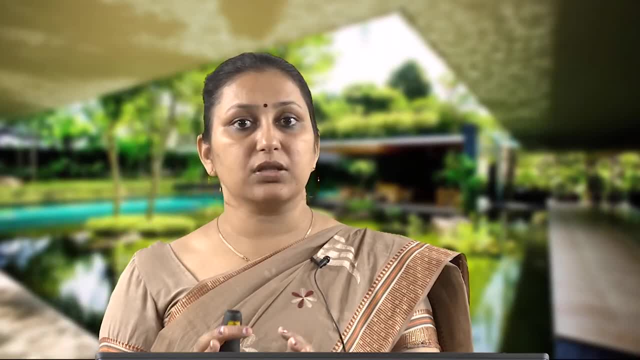 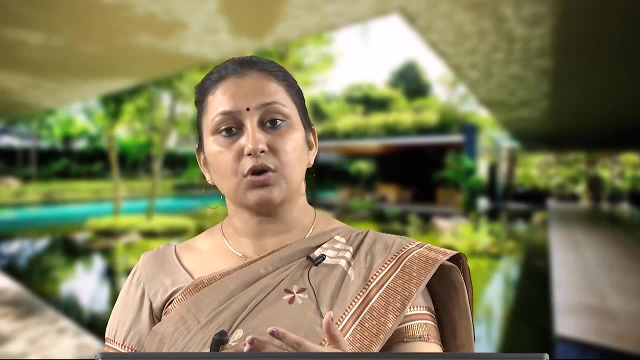 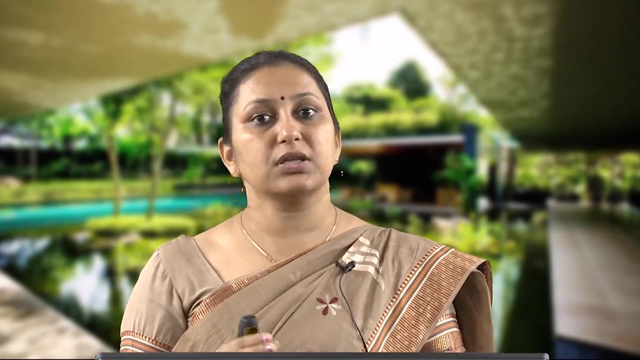 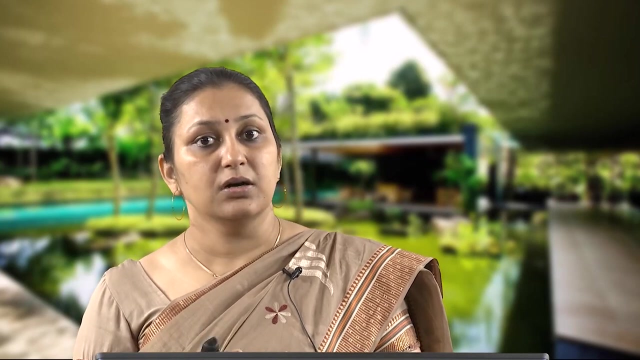 occupants. So only thermal comfort is not the one which should be considered or thought about while designing the buildings. it is also the visual and acoustic comfort. Visual and acoustic comfort find mention both in our history, in our codes like NBC, and also in our green building rating programs, the voluntary rating. 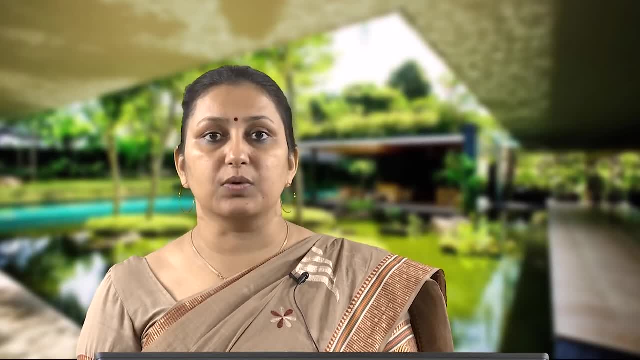 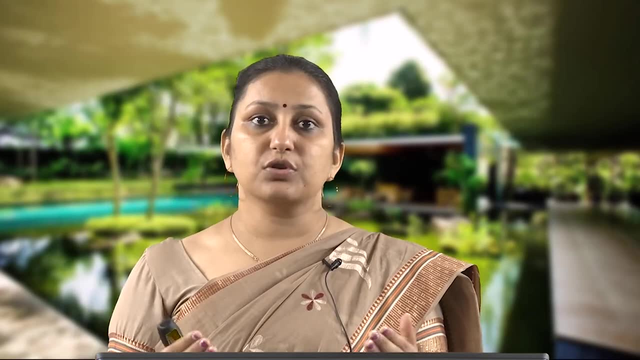 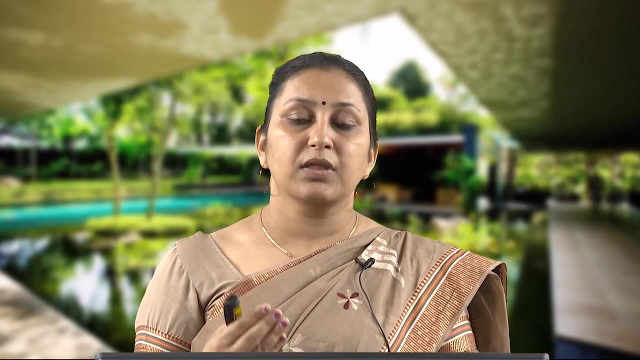 programs which are available. Let us quickly go over each of these and what are the related concepts and terminologies that we should be looking at. I am sure most of you have already undergone the courses on lighting and acoustics as part of your curriculum. 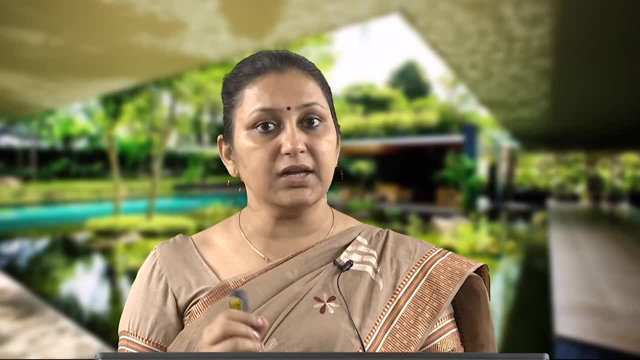 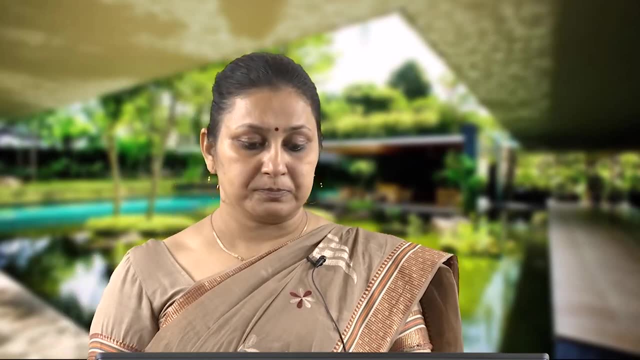 If you have not, some of these concepts are briefly introduced here, but not in great detail. So let us go over the visual comfort first. So what is visual comfort and what comprises of visual comfort? So there are many components to it. 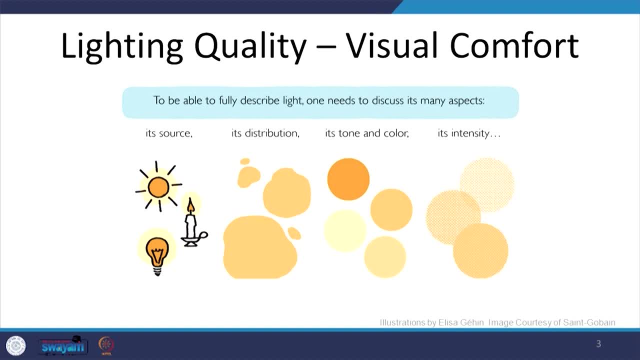 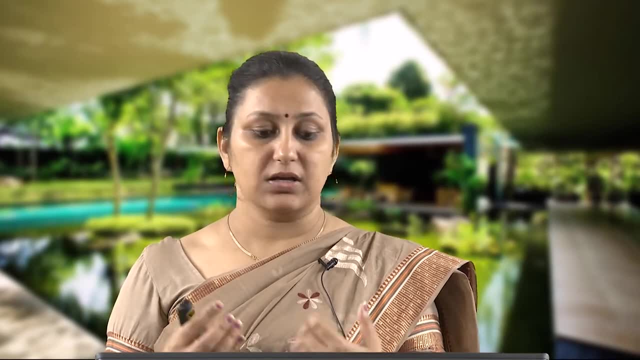 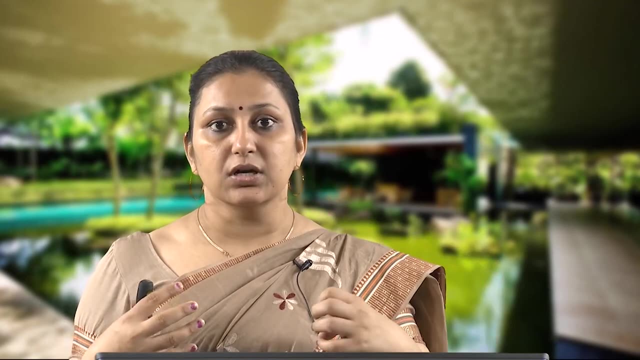 The first one, which is essential for visual comfort, is the source of light. So what is the source of light? The other which contributes to it Is: how is it distributed? So if it is distributed non-uniformally, so in one place, you have more light in the other place you have less of light, then this varying distribution causes discomfort. What is the tone and color of the light that we are using? So earlier people were using candles or flames for lighting up the interiors. gradually we moved on to incandescent. 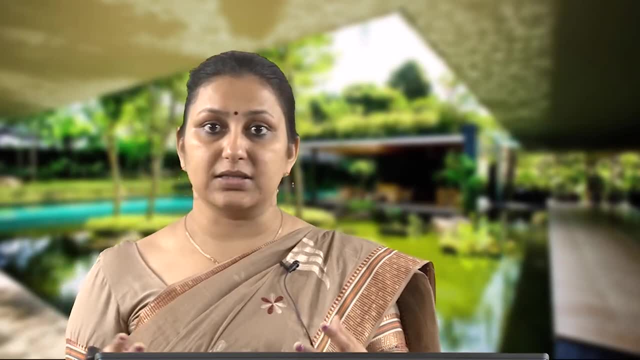 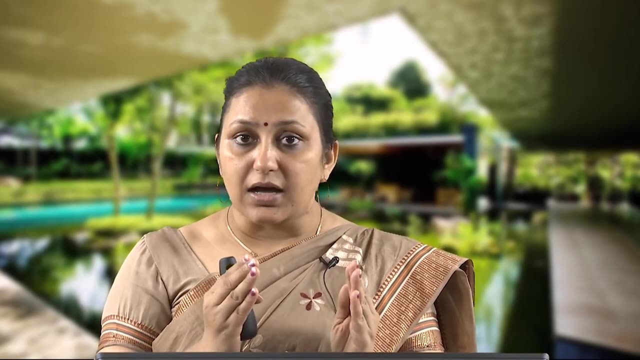 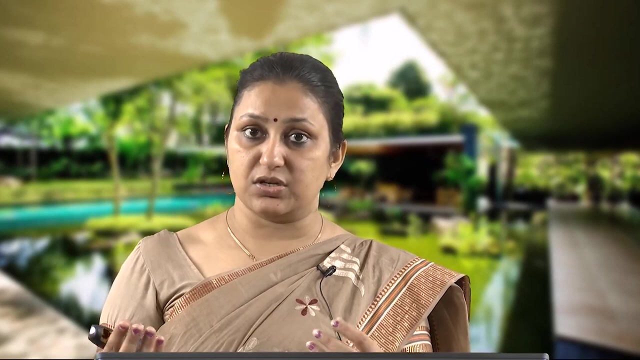 So what is the source of light? Incandescent bulb, and then we moved on to tube lights and now we are using CFLs and LEDs. as the technology has progressed, the quality of light, the tone of light, has also changed. So earlier we were using yellow light, where the color of the light was yellow, the tone 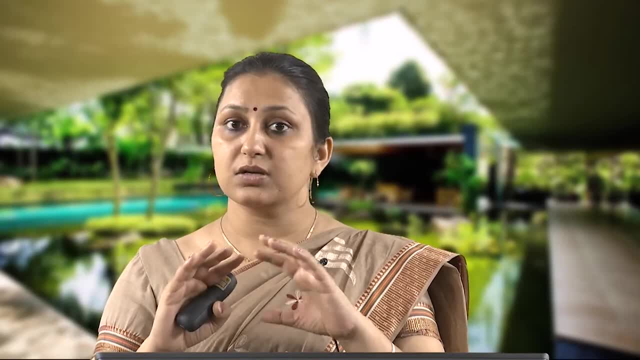 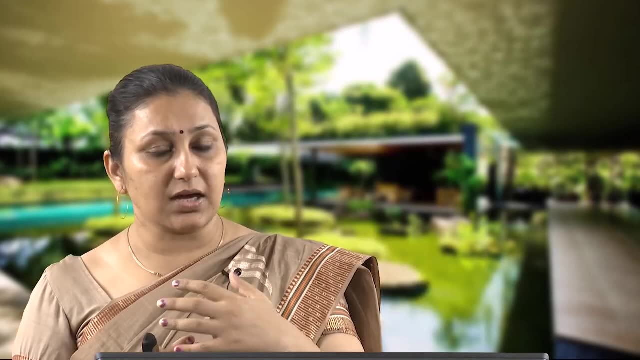 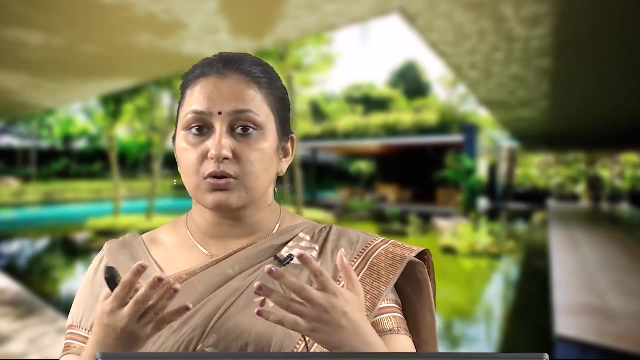 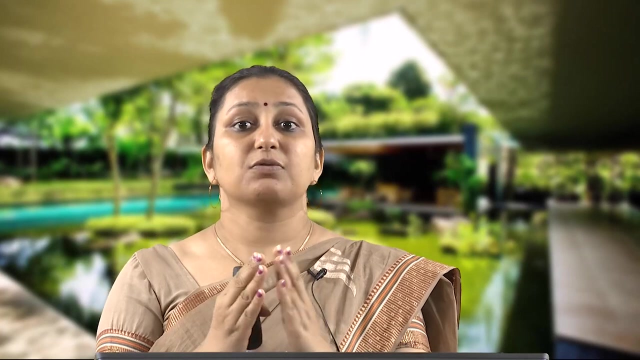 was such and gradually we are moving to more sunlit kind of light, the light, white light that we receive from direct sun. It is very similar to what we are able to produce using the artificial light as well. So, where there is a wide spectrum of colors available, where it is a white light, a combination, 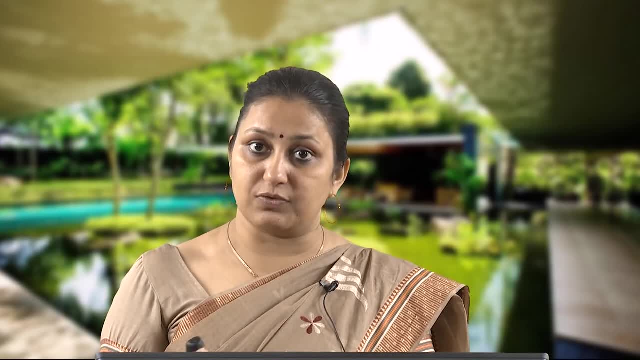 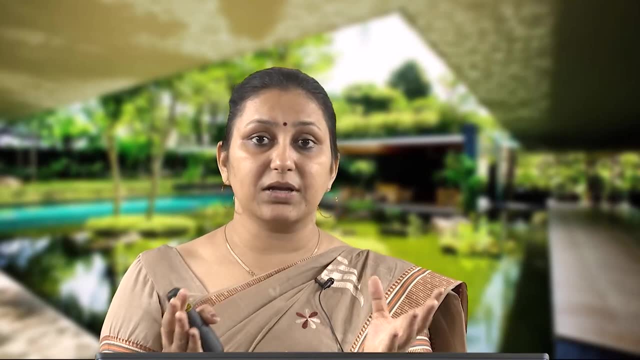 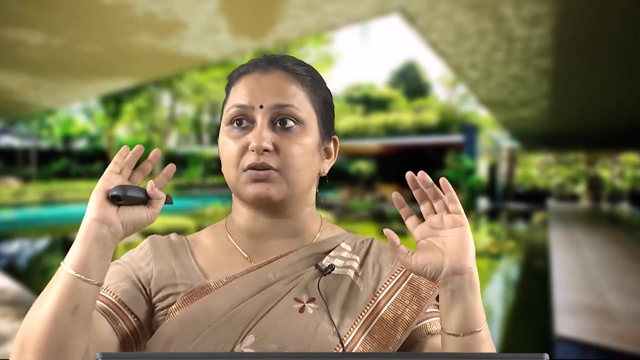 results in a white light is what a good color or tone of the light is. Wherever there is a different tone or color which is there in the light, it is not usually comfortable. So we are talking about long working hours. So suppose assume yourself working in a space which has only red colored lights all around. 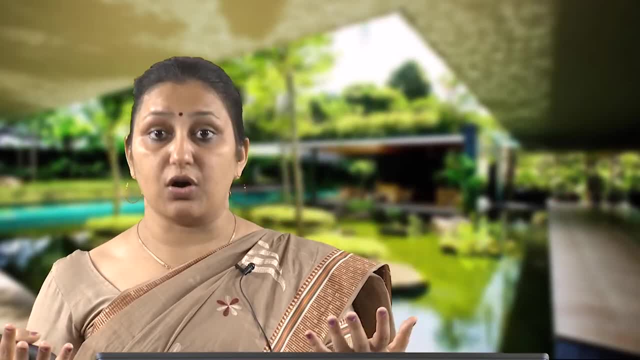 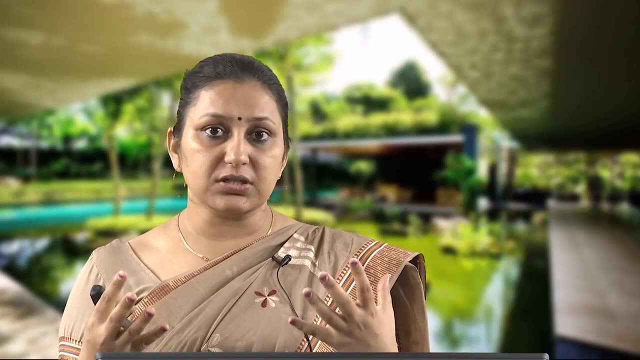 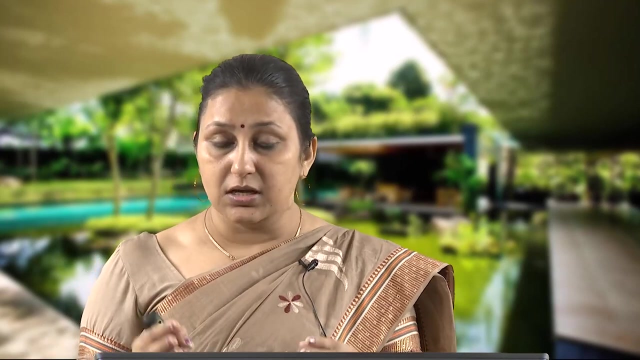 you. you will not feel comfortable for long sitting in that space. The last one is its intensity. So we need intensity sufficient enough to perform a task. Now that varies from activity to activity, space to space, depending upon the activity and the space the intensity has to be. 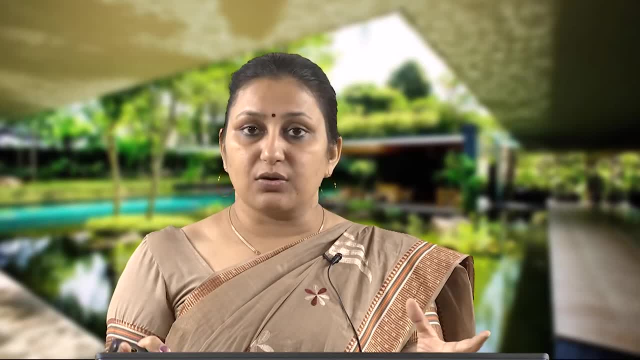 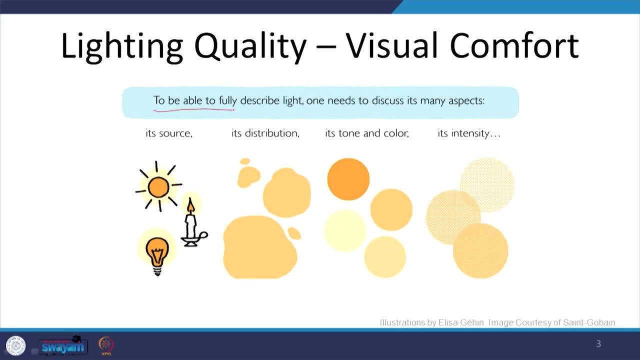 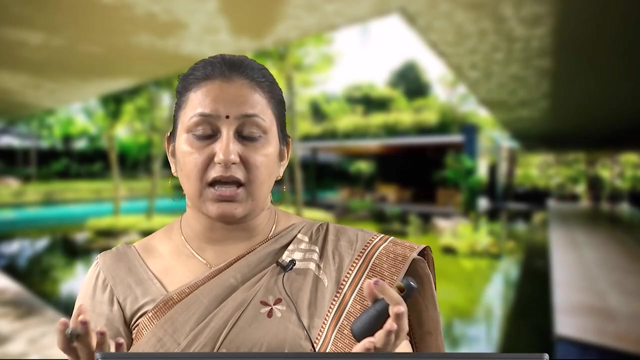 So we need intensity, So T cycles of light and space has to be there Together. all these four parameters define what visual comfort is. Visual comfort is defined as the ability to fully describe light and understand the space as it should be perceived or as it is. 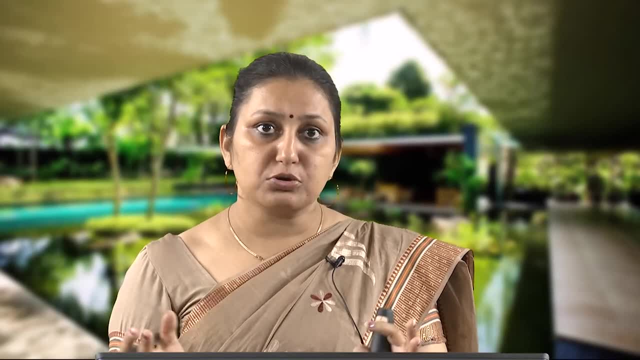 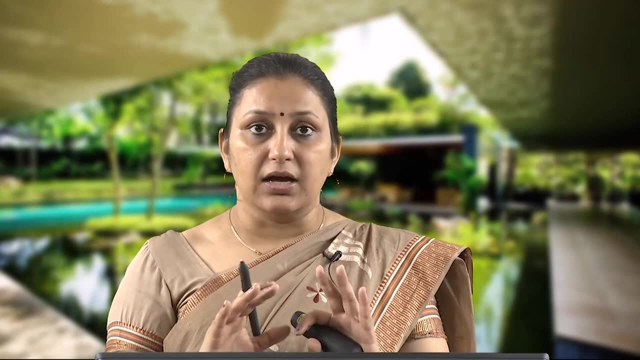 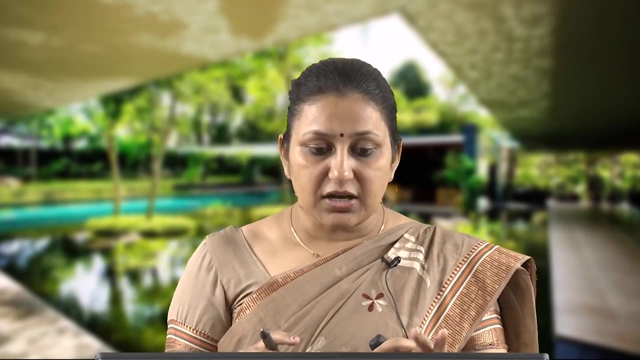 So it is the absence of discomfort because of its source, distribution, the tone and tone and color and its intensity, and the absence of this discomfort is called as the visual comfort. So when we are talking about visual comfort, we are talking about two aspects: the quality, 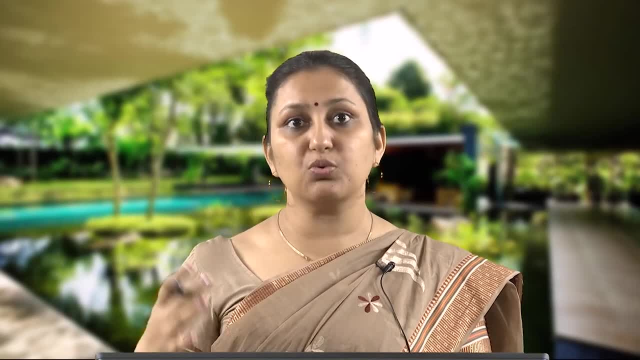 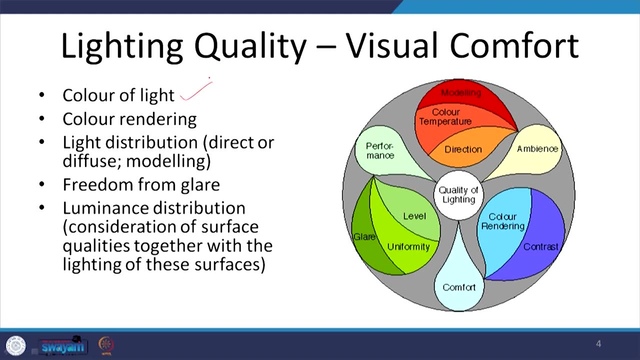 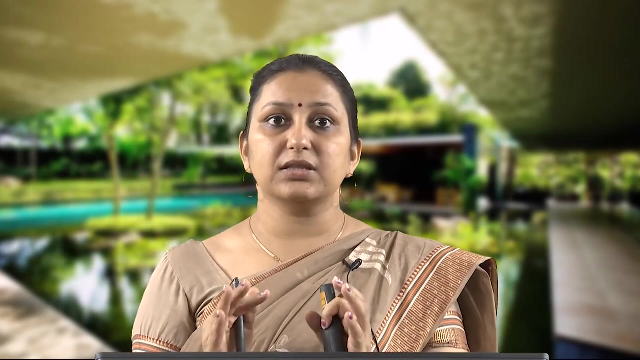 as well as the quantity. So of these four parameters, two are used to define the quality of it. First is the color of light. as I just said, that color of light defines how comfortably things can be seen in the given light. preferably, the light color should be close to what the 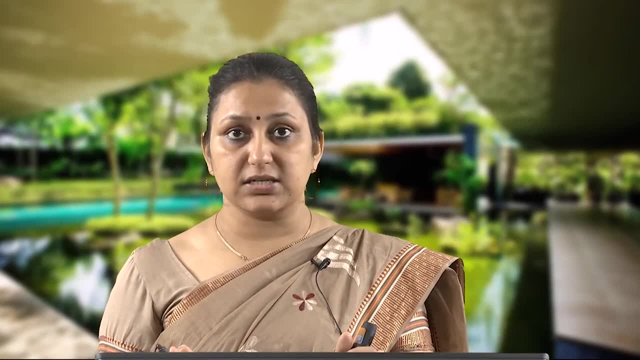 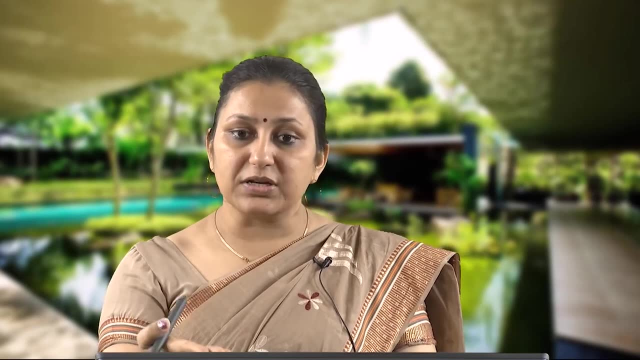 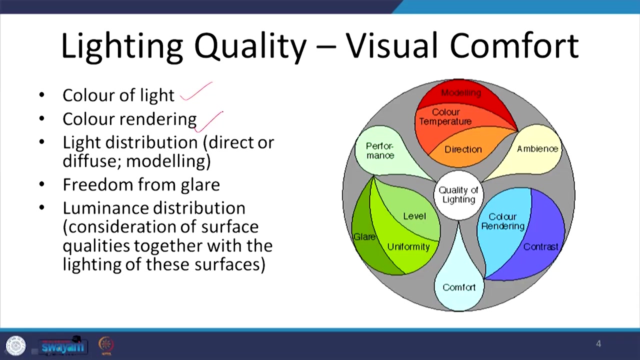 color of direct sunlight is, which is white. We should comprise of all the colors equally and we should be able to perceive the color of any given object as its original color, and that is what the color rendering is. So here we are, looking at the light. 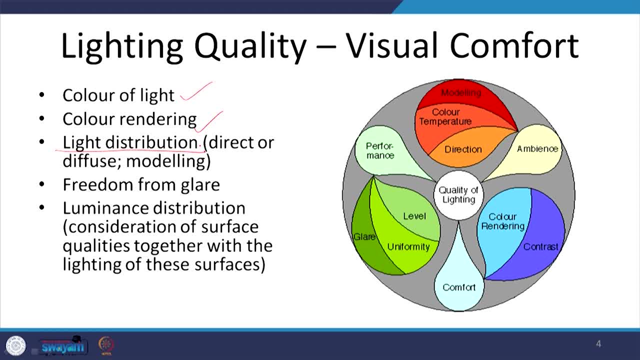 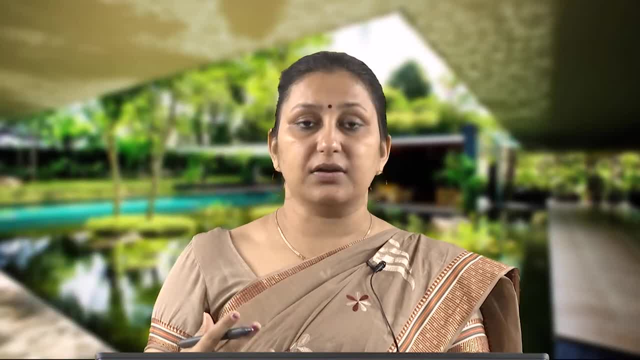 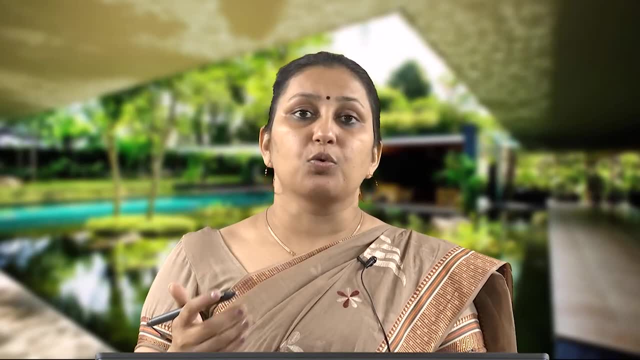 Light distribution also, which is direct or diffuse. now suppose I have a lamp right on top of my head, So there is direct light there, while if I have a, in case of artificial light, I am saying in case of a bulb, where I have a diffuser, where I have a reflector which reflects it, 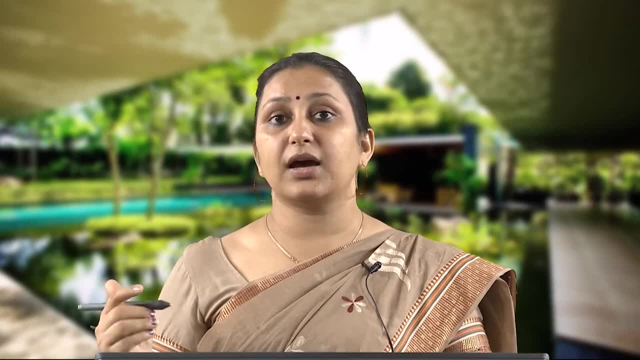 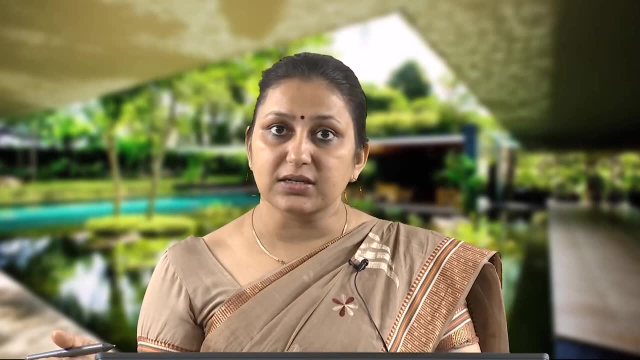 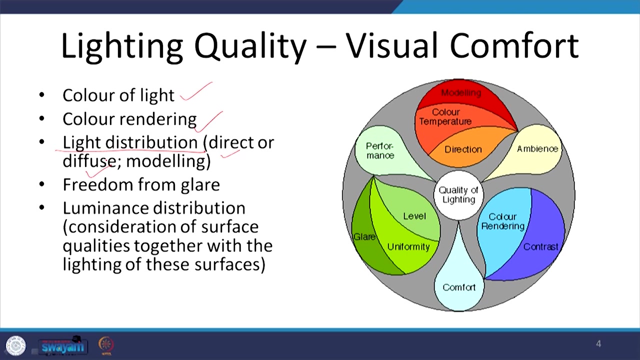 to the ceiling, and then I get diffused light where I do not get any shadows, I do not get glare. Same Same for artificial as well as natural lighting. So what kind of light distribution is there, whether it is direct or diffuse in some cases. 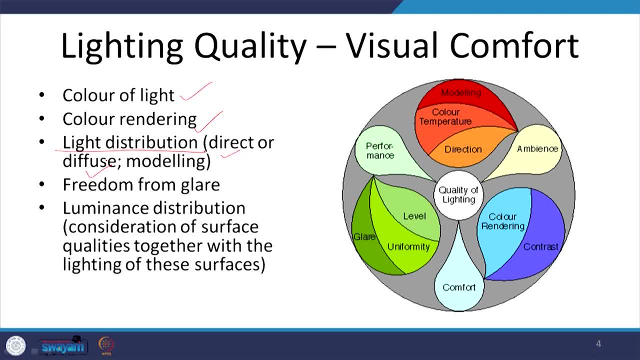 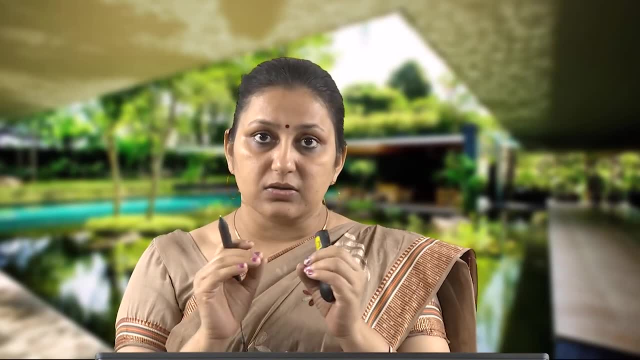 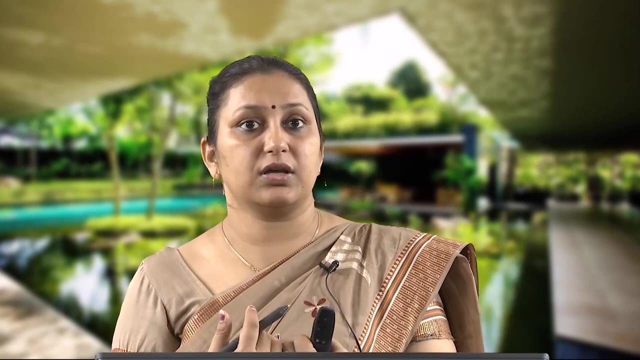 direct light is required, For example, for a doctor who is performing a critical operation in the operation theater there. he may want to have there. we may want to have direct light focused onto the operation area where the doctor is able to clearly see things Because he is going to perform a critical operation there, unlike when we are working. 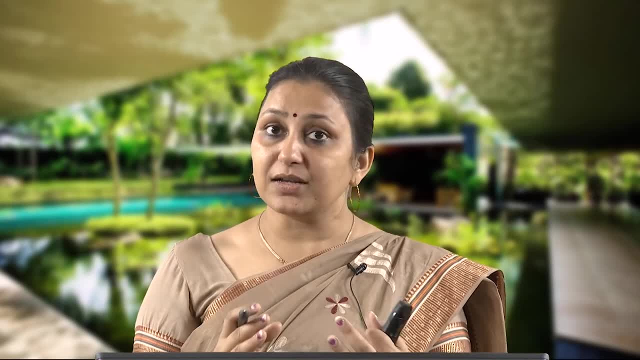 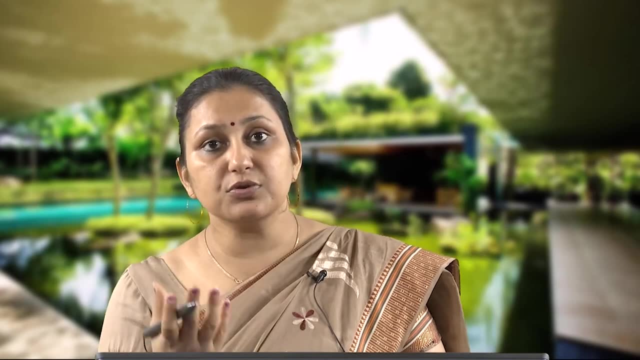 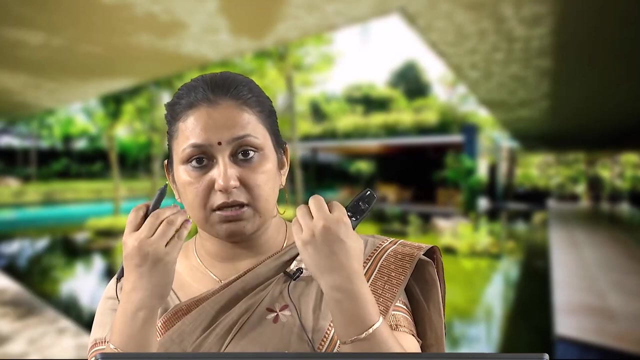 or when we are reading in a classroom. there I might not require direct light falling onto my book, onto my notebook. I would prefer diffused light, because I have to sit looking at my book for long hours and there diffused light would help keep stress off my eyes. 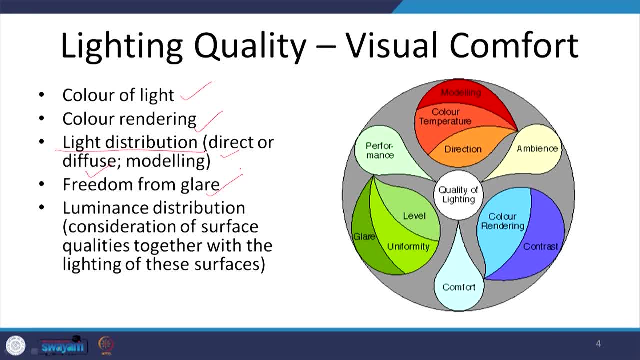 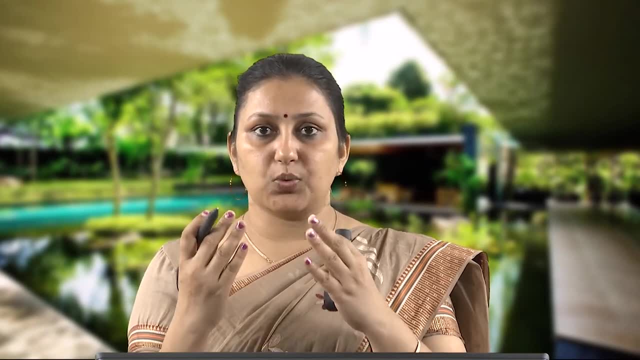 Another thing that we require here is freedom from glare. We will come to glare, what glare is, in subsequent slides, but glare is that pinching light directly falling onto your eyes. It is not necessarily the direct light, but it is when there is a great difference between. 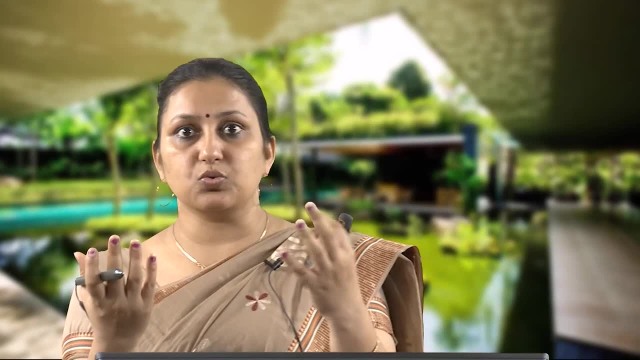 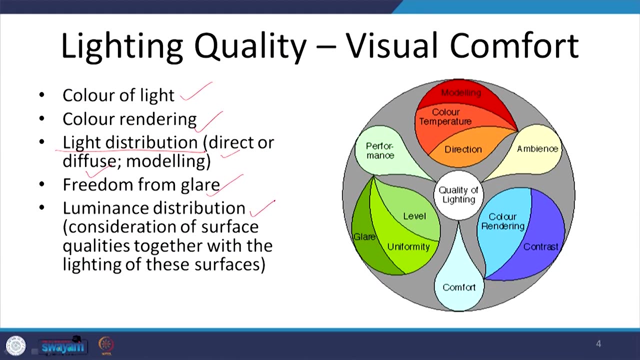 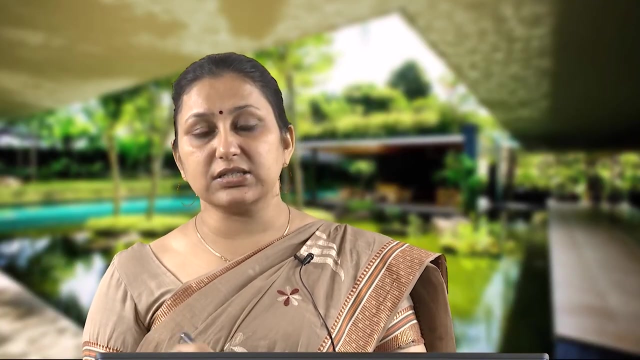 what my eyes are used to, and suddenly, when I go into a bright light, or there is a bright light coming from somewhere, So we are looking at the luminance distribution, how the luminance is distributed throughout the work surface. So these are the qualitative aspects of visual comfort. 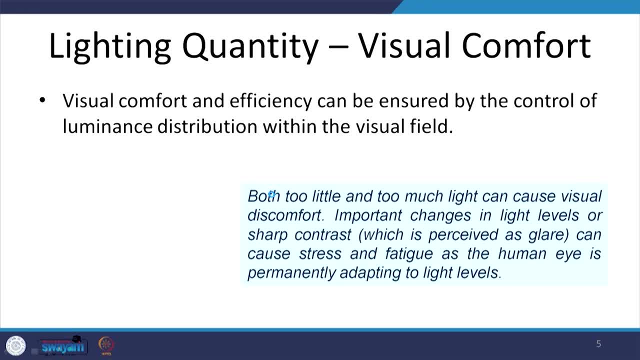 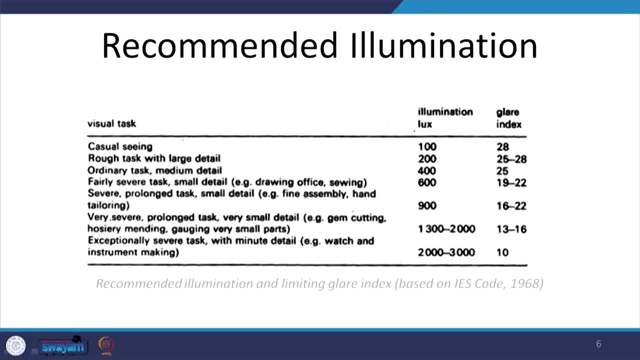 We are also looking at the quantitative aspects of these visual comforts. Some of these qualitative aspects can be converted into quantities. So first of all, we are looking at the illumination: how much of the light, the intensity, is going to be there. So when we are talking about illumination, we are talking in the units of lux and for. 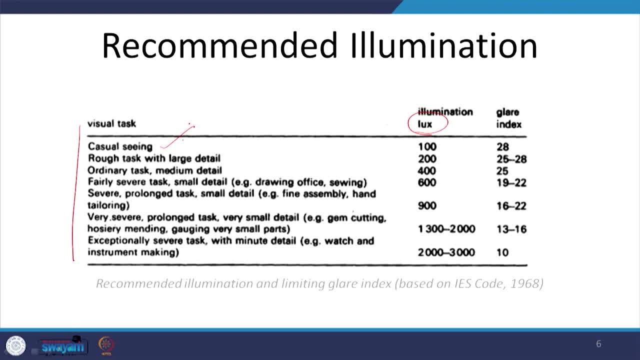 different types of tasks, from casual seeing to exceptionally severe task with minute detail. as I was talking about the operation theater, the illumination level goes on increasing. So if we are casually walking around seeing things, a 100 lux illumination is sufficient enough. 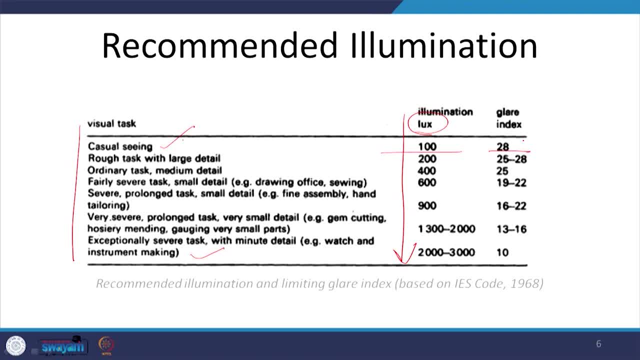 So even a glare index as high as 28 is also fine, because we are casually seeing around things. However, when we go high on the intensity of the visual task, for example, we look at the ordinary task or medium detailed task, which is where our classrooms and offices 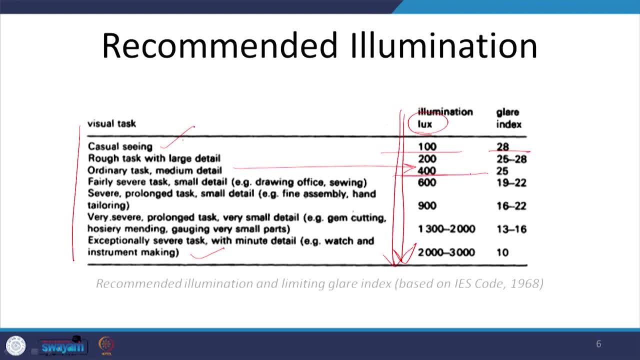 come in, We look at an illumination level of around 400 lux- 400 to 500 lux is what we would want In our offices and classrooms- and a glare index of around 25, we will come to what glare index is If you look at very severe or prolonged tasks which require minute detail, for example, gem. 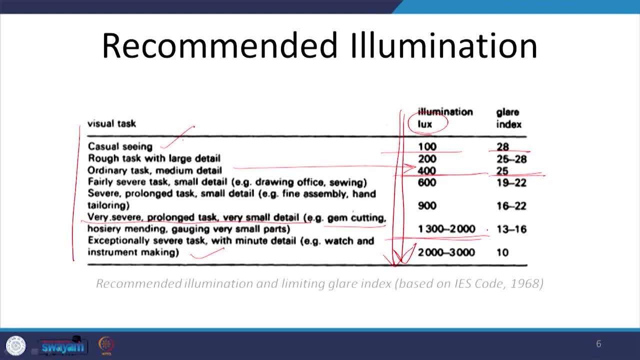 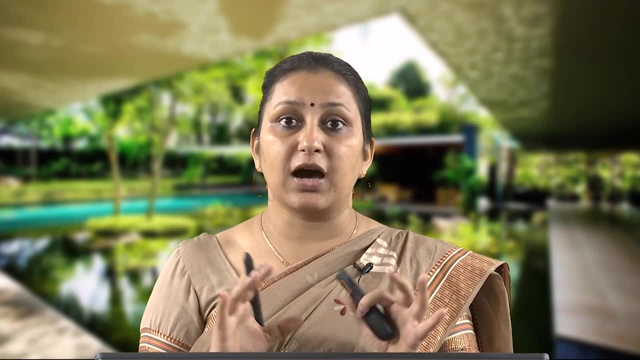 cutting there. the lux levels are quite high, but though the lux levels are high, we are not promoting a very high, We are not accepting a very high glare index. the glare has to be less, So the entire workspace has to be highly lit, along with the task table. 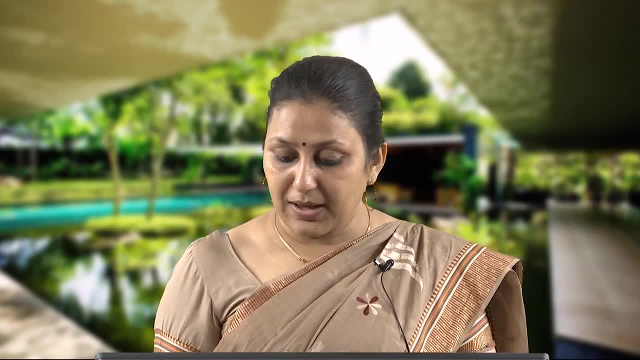 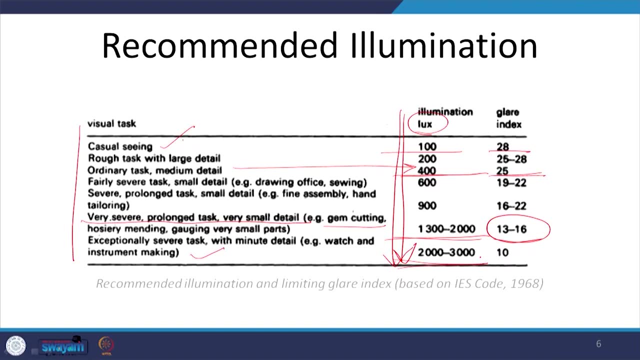 along with the task work plane And the maximum. it goes up to 2000 to 3000 lux, which is in case of operation, theaters or instrument making, watch making, which is very minute. very small parts go in and the glare is further reduced. If I look at beyond the quantity quantitative, 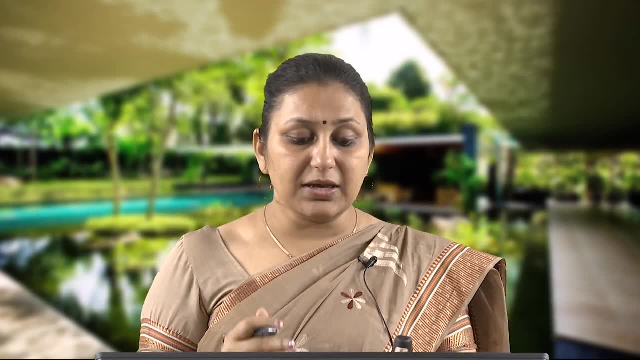 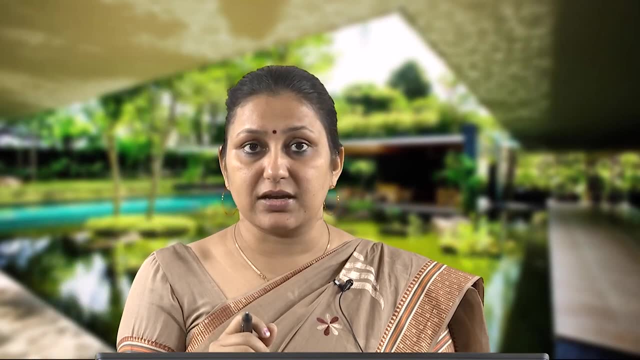 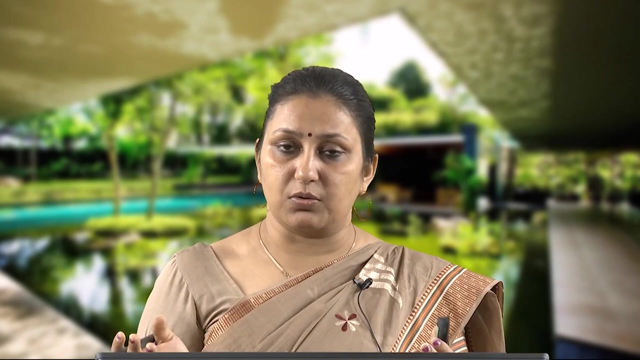 aspects of visual comfort. in general, the ability to control the light levels by the occupant is key to the satisfaction. So suppose I am in an office area where I cannot control the illumination around. Today I might be feeling a little low and I might be feeling a little low. So I am in an office area where I cannot control the illumination around. Today. I might be feeling a little low and I might be feeling a little low. So I am in an office area where I cannot control the illumination around. Today. I might 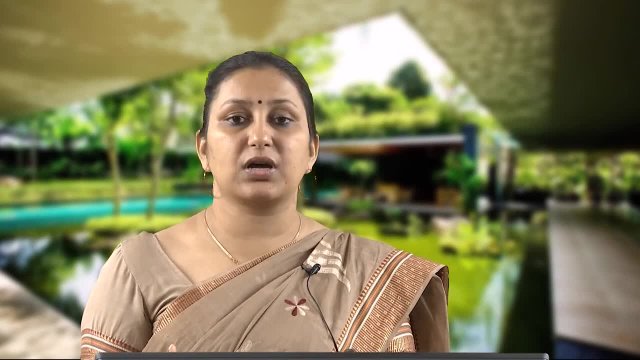 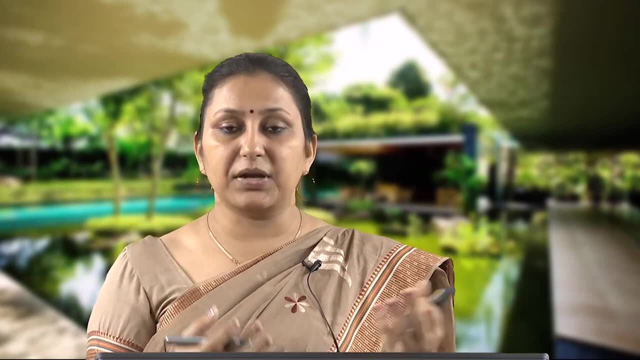 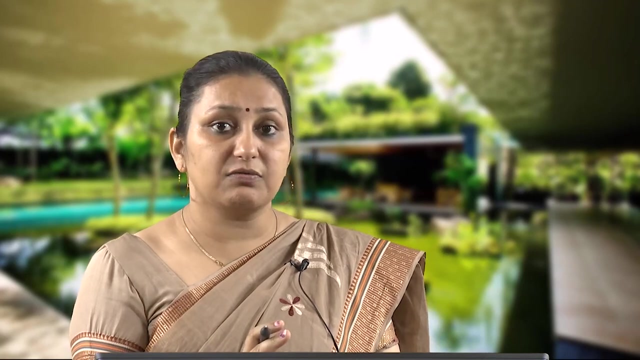 require more light to perform a task- the same task as compared to some other days where I might want to work with less of the light, depending upon my mood, depending upon my comfort. That ability, that flexibility in the built environment is also a key to satisfaction. 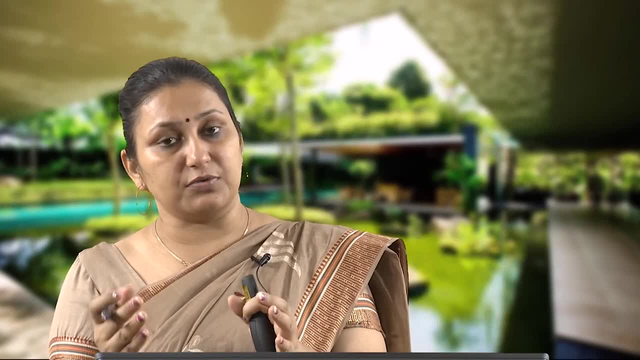 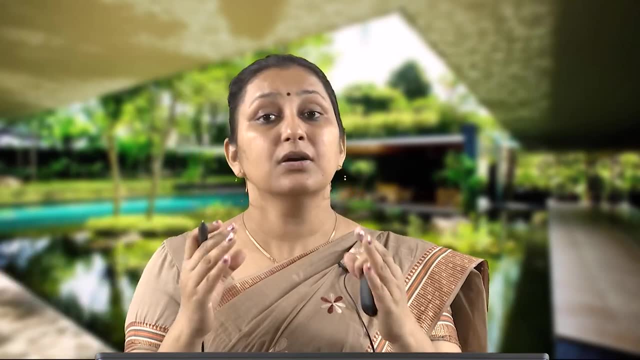 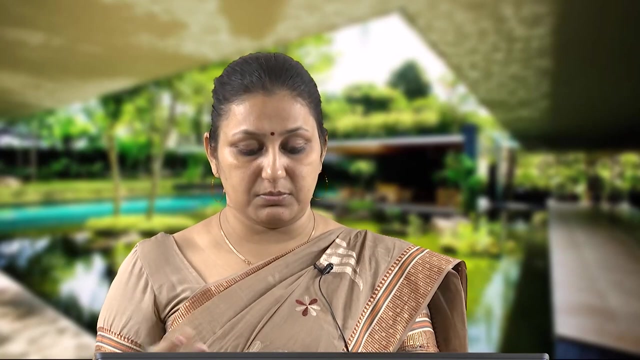 So it is both for thermal comfort, for visual comfort. equally, If I am able to control my thermal environment and if I am able to control my visual environment, the researchers have proven that the occupant is more likely to feel comfortable, be at comfort. 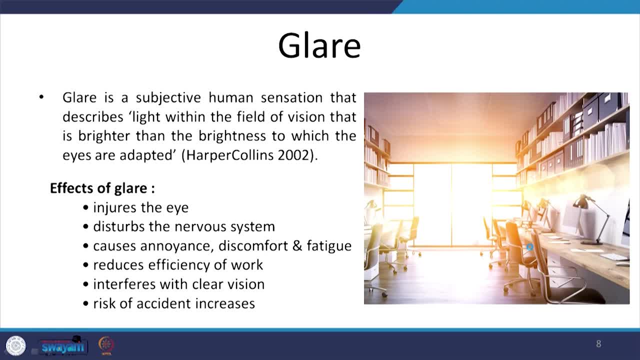 Now we come to glare. So glare, as defined, is a subjective human sensation that describes light within the field of vision that is brighter than the brightness to which the eyes are adapted. Now, this brightness to which the eyes are adapted is the overall brightness of the place, The general 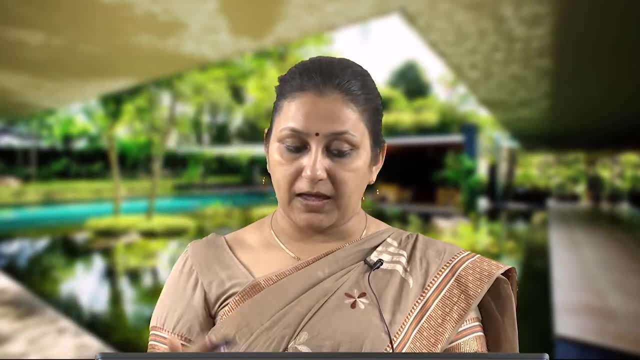 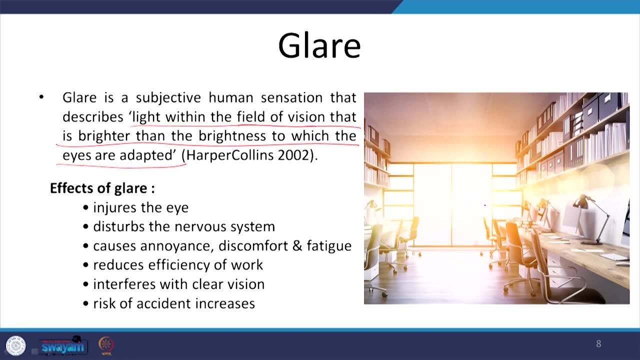 illumination level, illuminance of the place and the light within the field of vision. So suppose I am sitting here if we look at this, this picture, So if somebody who is sitting here is usually looking at this wall, this is the work side, this is the work desk and this side is where 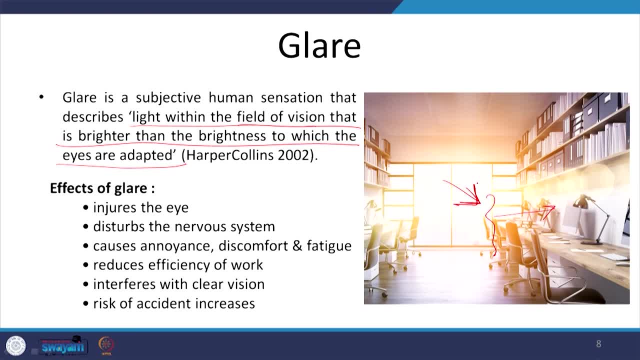 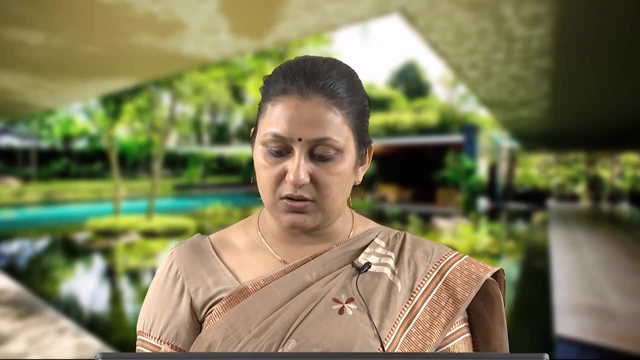 the bright light comes in. So the difference between the brightness coming from this side versus the brightness which is prevailing in this larger area- this is the brightness which is prevailing in this larger area versus the brightness which is prevailing in this room- is what is perceived as glare and there are quantified formula to define. 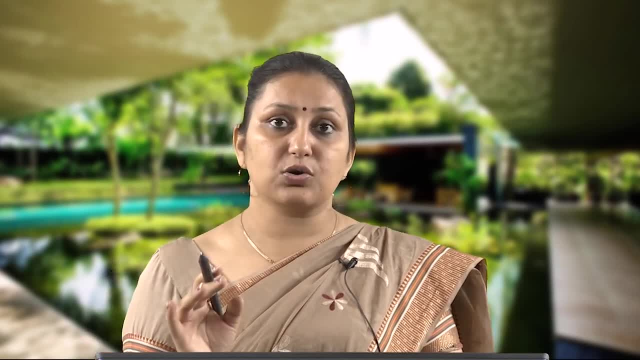 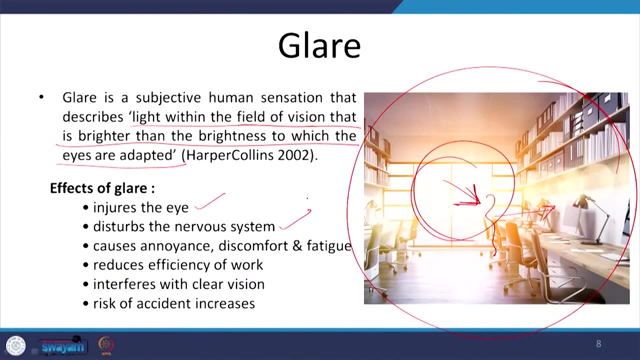 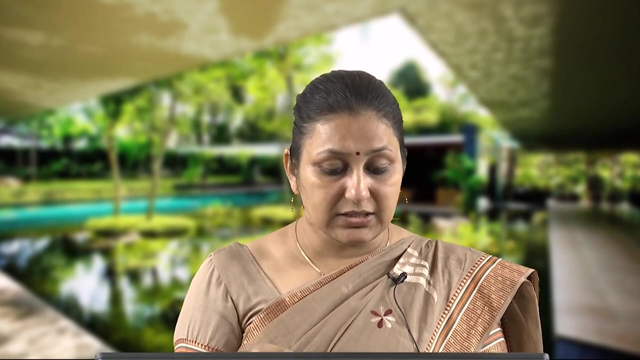 what glare is. but glare is often harmful because it injures the eye, it disturbs the nervous system and at times it when we are talking about injuring the eye. it almost blinds a person. you cannot see. It is a cause of annoyance, discomfort and fatigue. So if you are 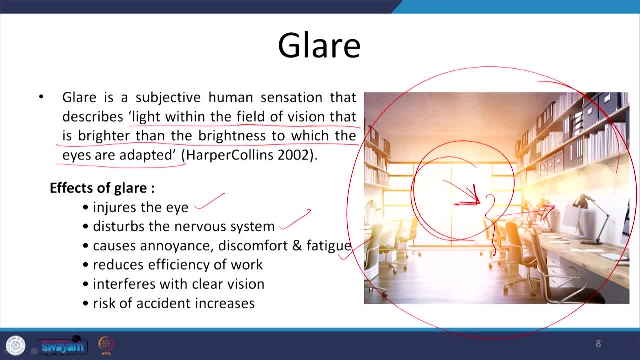 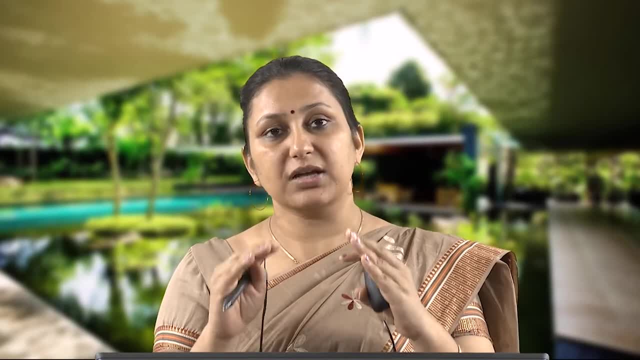 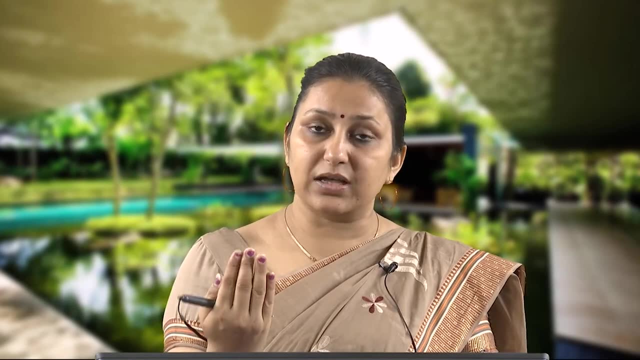 constantly, for example, if you are driving during the night and there are vehicles coming from the opposite direction, So your eyes are used to a much lower level of brightness because it is night and suddenly, when the light from the vehicle which is coming from opposite side hits your eyes, 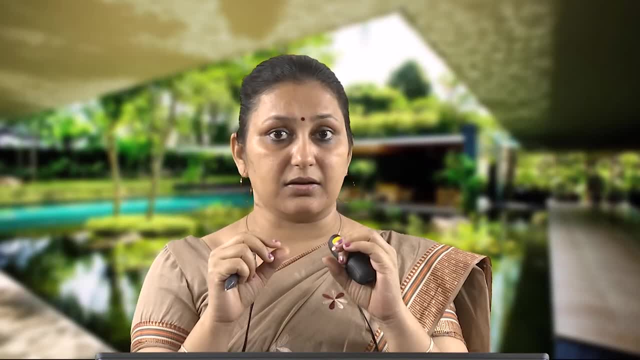 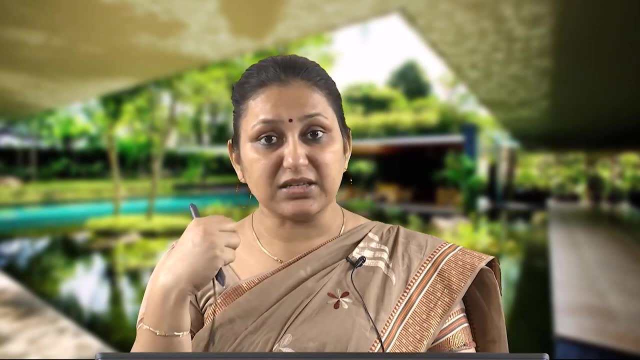 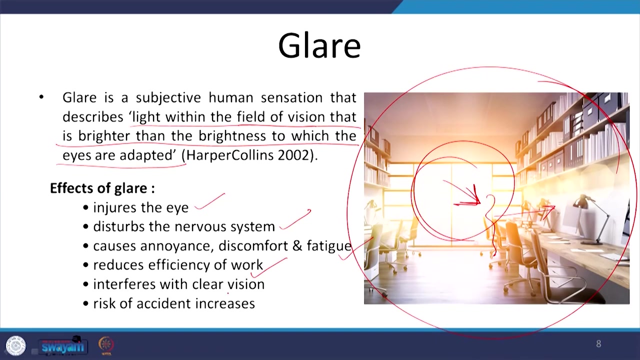 that is what causes a discomfort because of glare. Now, constant exposure to this glare causes fatigue. It is mental fatigue, it is fatigue to eyes, it is fatigue to body. So it reduces the efficiency of work and it interferes with a clear vision, which is 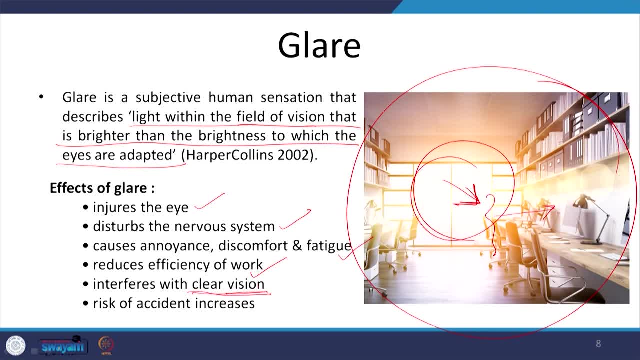 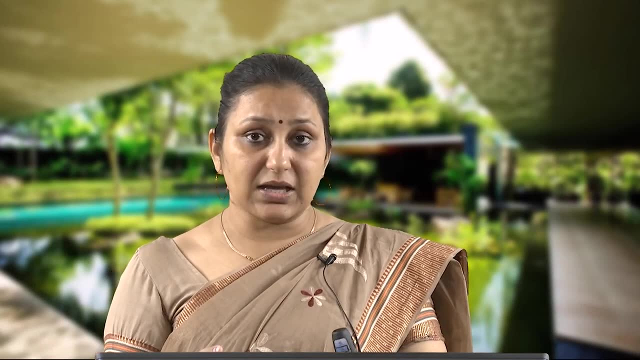 what I say, that people are almost blinded when there is glare, when there is high glare, and thereby increasing the risk of accidents. So a lot of accidents happen because of this glare on highways. So I am giving example of glare from highways. 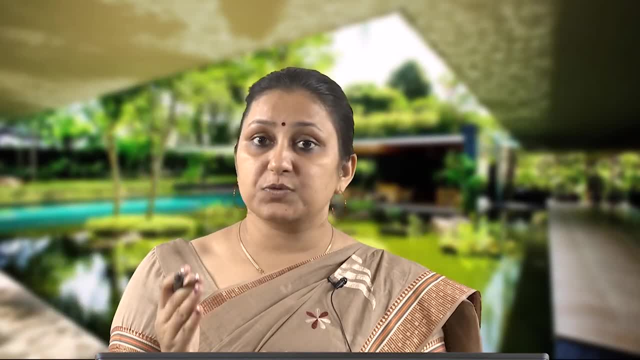 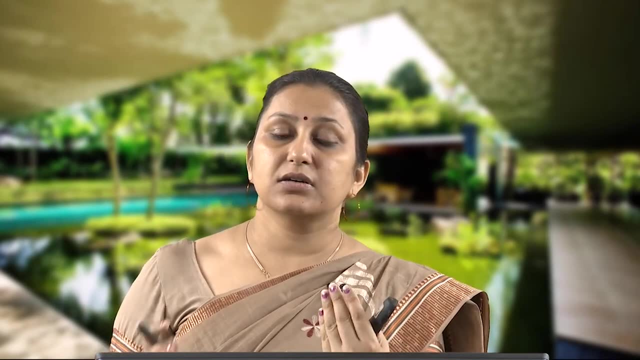 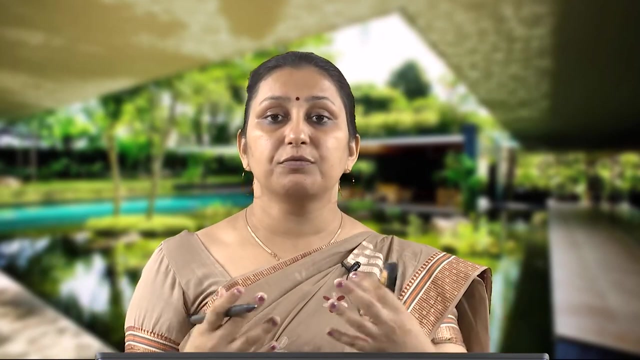 but when we talk about the buildings, we experience a lot of glare coming because of surrounding buildings. So suppose I have a window and there is reflection coming from the building which is adjacent because of the light colored finish of that building. a lot of reflection. 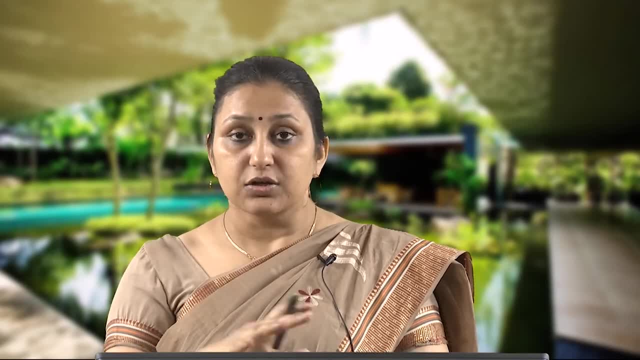 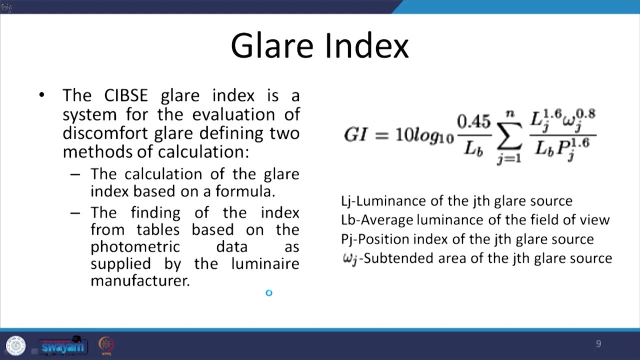 of light is coming onto my window and onto my eyes, So that is how the glare inside a building often comes in. To define glare, the glare index has been defined, which is what we just saw when we were defining the illumination level and the glare indices. So the formula incorporates largely the illuminance. 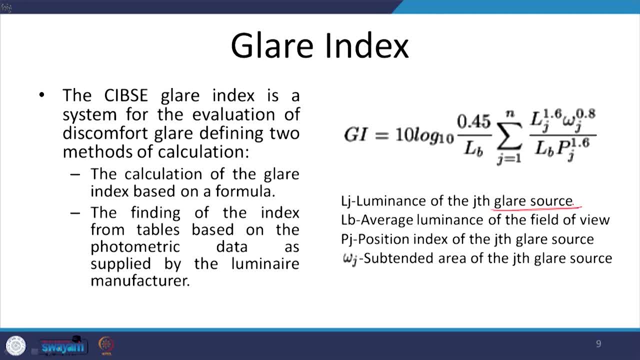 of the glare source which is under question. the average illuminance of the field of view to which the eyes have adjusted. the position index of the glare source, how far or how close it is to the mirror. The object to the area under study- subject under study and the subtended area of the 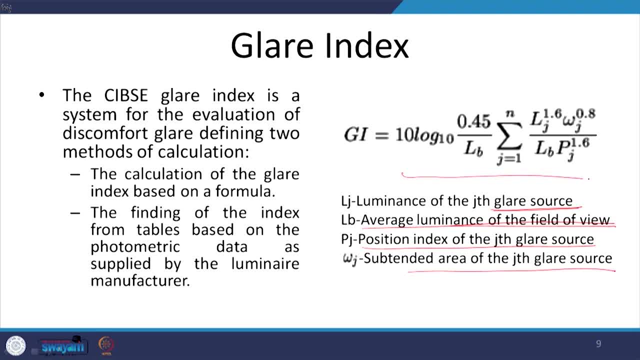 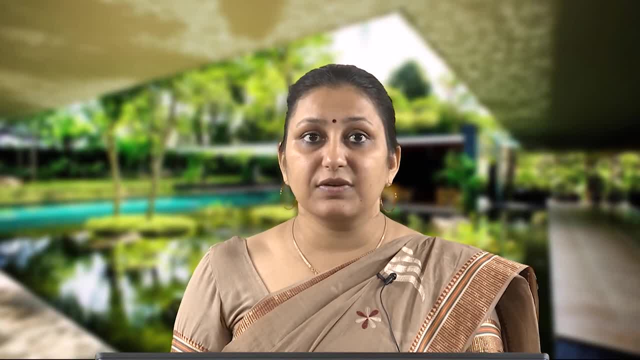 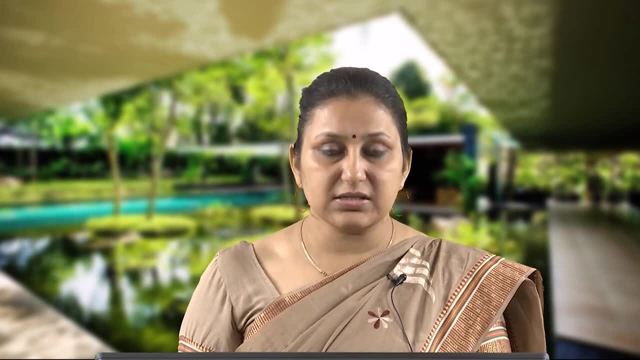 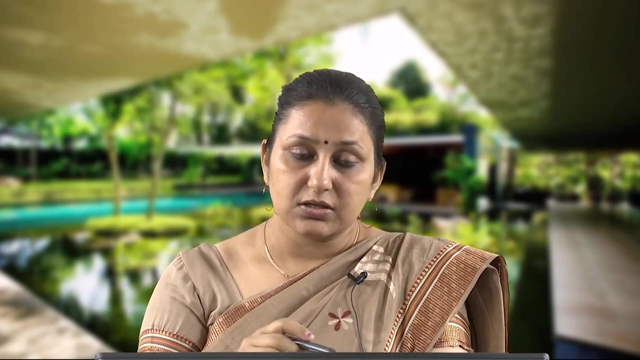 glare source. put together in a formula, it gives us the glare index. With the help of this glare index, as we have already seen, we can define how much of glare is ok. So up to 25 is maximum that can be seen. That can be accommodated. this is as per CIBSE glare index, but there is a new glare rating. 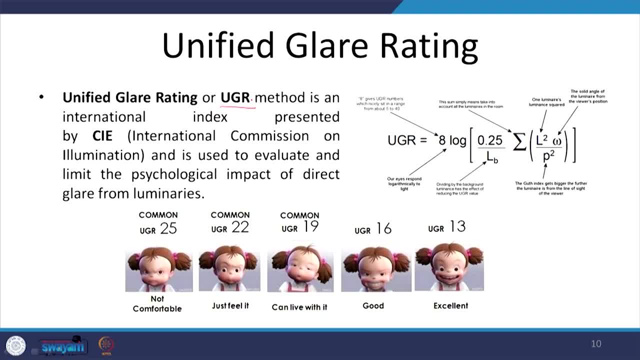 which is unified glare rating, or UGR, and it is defined by this formula again, where we are taking into account the background luminance, We are taking into account the luminance of the source and the luminary and putting together in a formula, in a formula to get the UGR. So 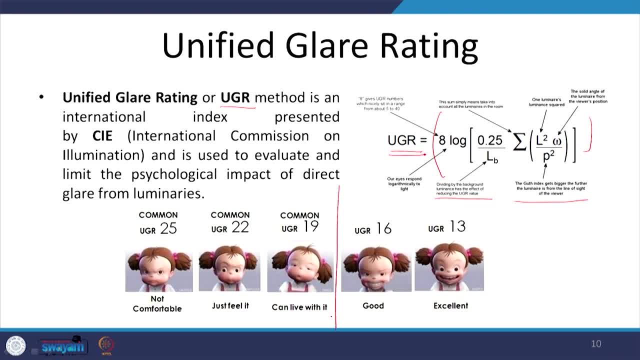 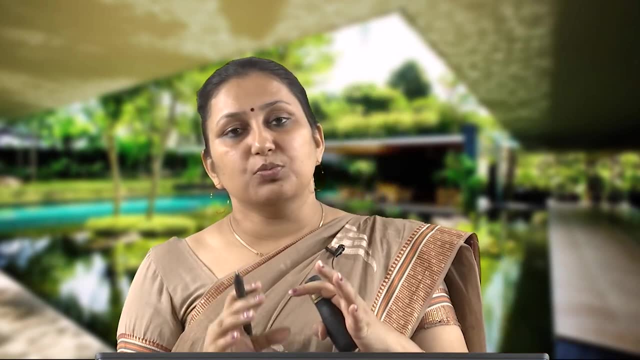 As per the UGR, we are looking at a limit of UGR 16, which is good enough for the human eyes. beyond 16, it is not advisable to have the glare Now, when we have talked about the illumination level, the illuminance and the glare index, 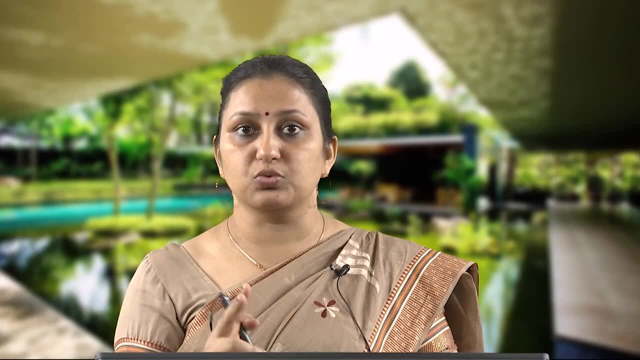 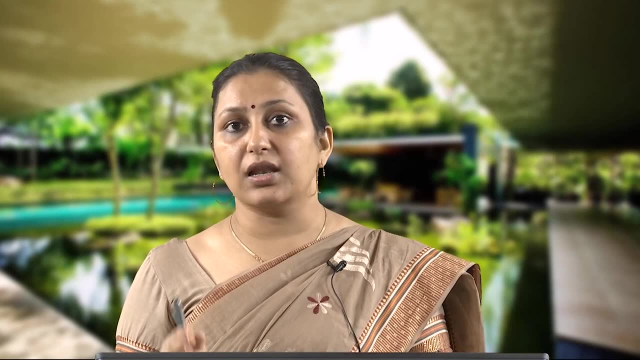 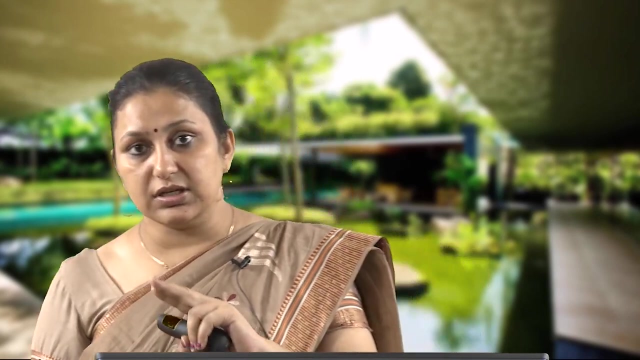 always, whenever we are talking about visual comfort, we are talking about two things. We have to look at strategies to control glare and to allow for this minimum illumination which is desirable. Besides these two, the qualitative parameters, where we were talking about the color of light. 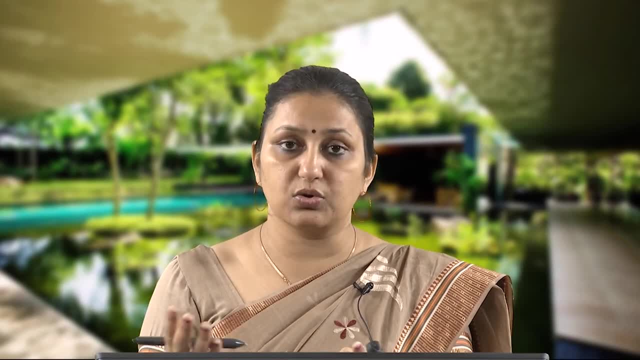 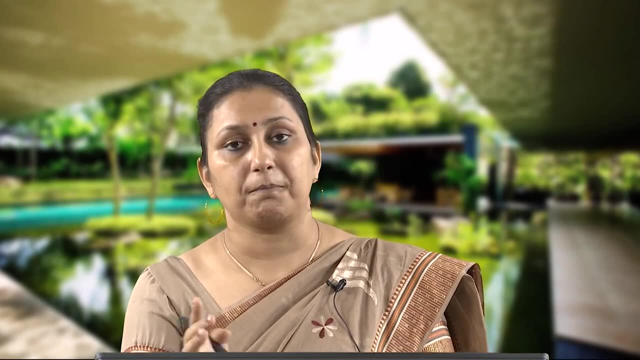 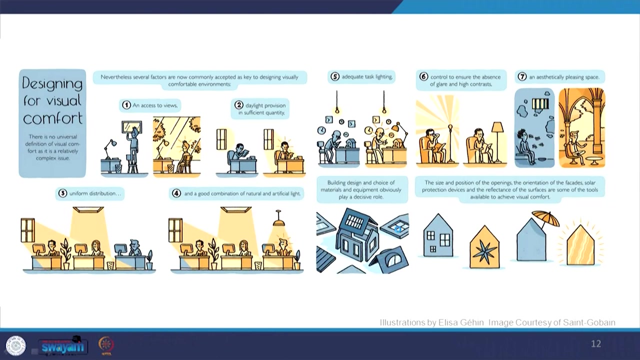 and we are talking about the uniform distribution. the tone of the light, the tone, color and uniform distribution also comes into picture. And one more thing, which is The direct access to views. So how much can we view? So this is a beautiful illustration which is put up by Elisa Gahan, and it is available. 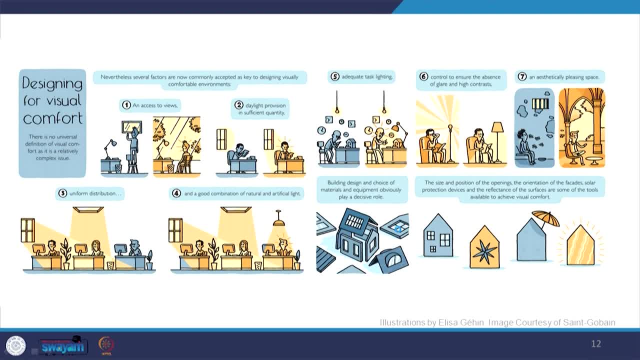 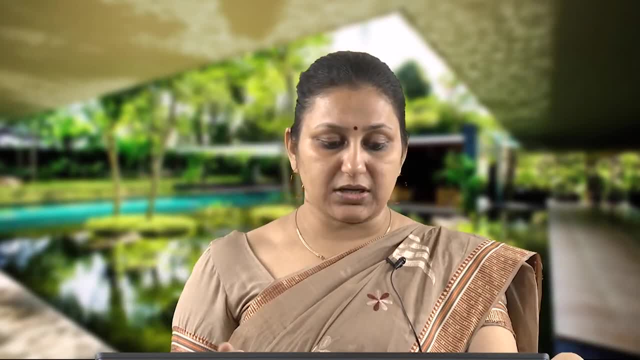 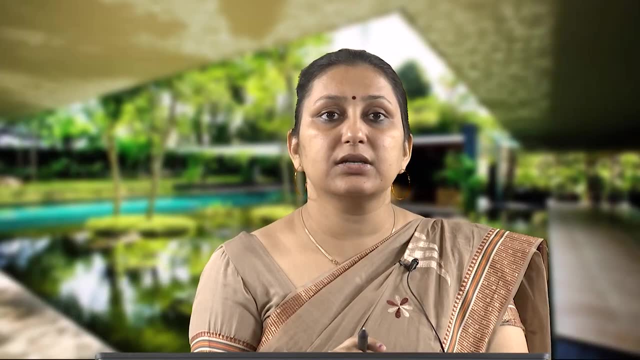 in public domain at the Saint Gobain website. So there are 6-7 strategies or indicators to assess visual comfort. First of all, which we often neglect, is an access to views. This is very well taken care of. We take care in green buildings, in sustainable building, where each workplace should have. 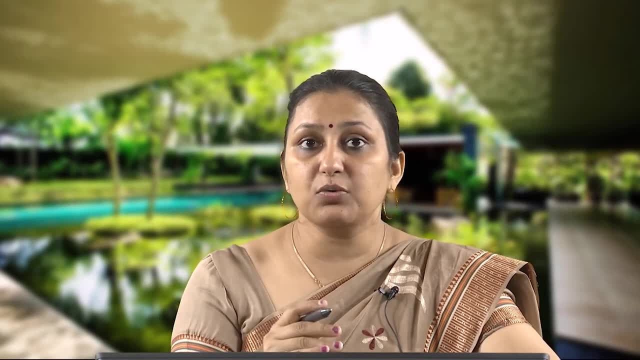 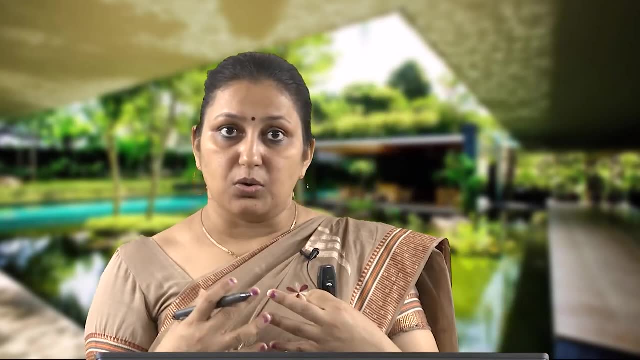 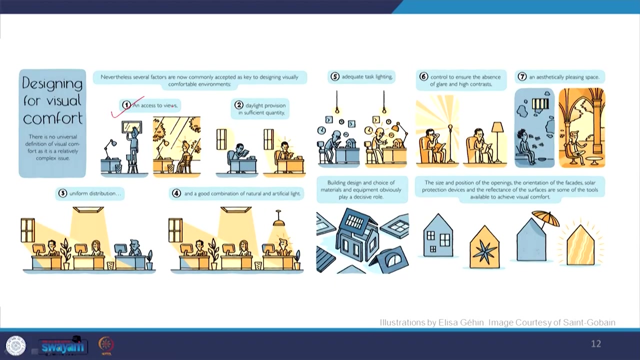 an access to views. If every workplace cannot be connected to the outdoors, outside the building punctures or green areas, natural areas within the building have to be created in order to provide for these views. The next is provision of sufficient daylight. Every workplace should be daylit as much as possible, though we may have sufficient. 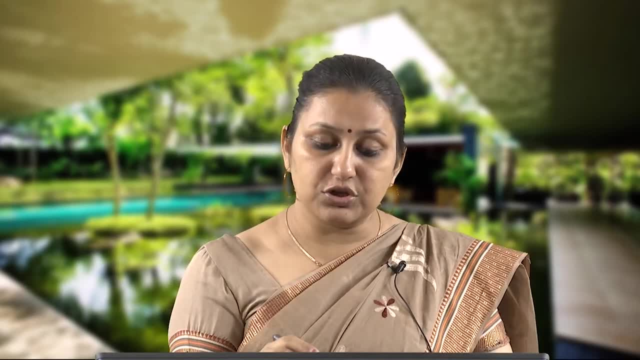 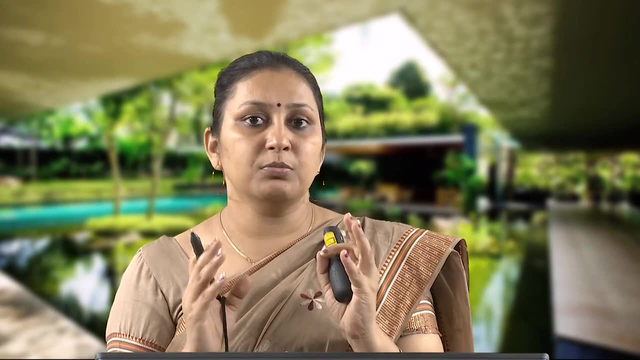 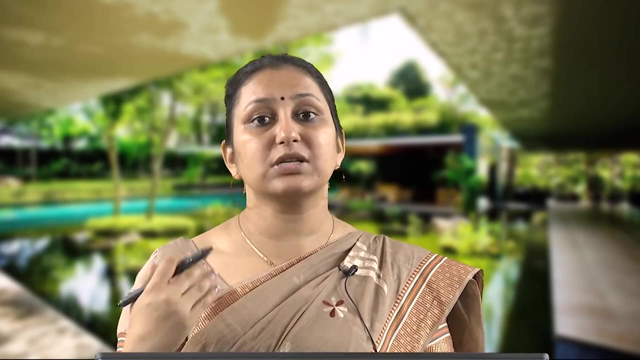 light available artificially. yet the provision of daylight has a lot of impact. Now we may not be able to perceive that immediately, but if human beings are continuously exposed to controlled environments where they cannot see the daylight, there are psychological changes which occur. 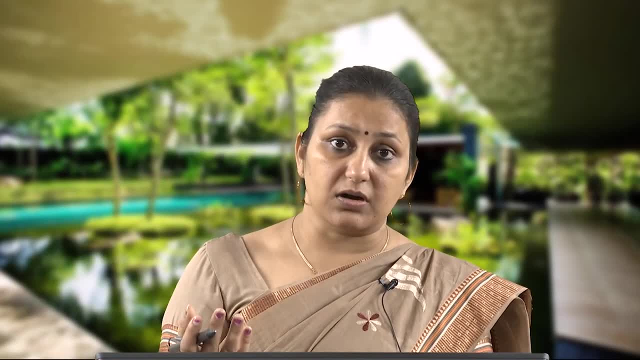 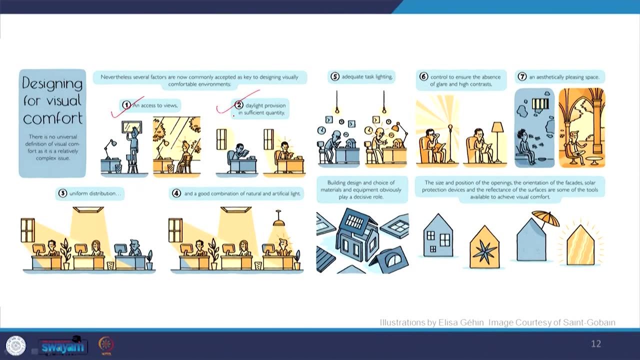 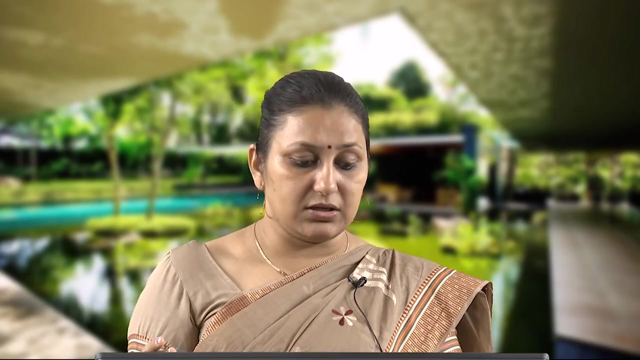 Right, Which start to happen, which are visible, and a lot of medical researches prove that. So direct provision of daylight in sufficient quantity is required for visual comfort. The next is uniform distribution of that. We cannot have some workplaces with limited daylight availability and others with less. 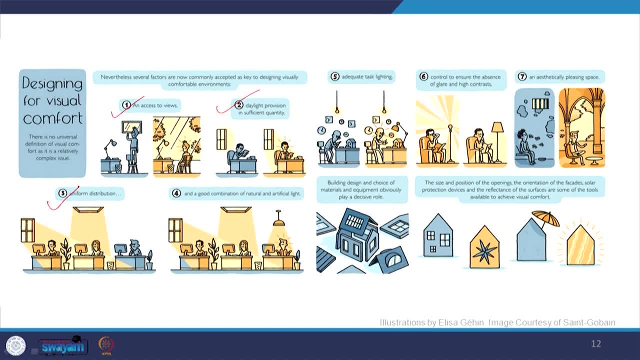 of that. If it is a uniform distribution, that is what will lead towards the visual comfort. So the next is uniform distribution of that. We cannot have some workplaces with limited daylight availability and others with less of that, So the next is uniform distribution of that. 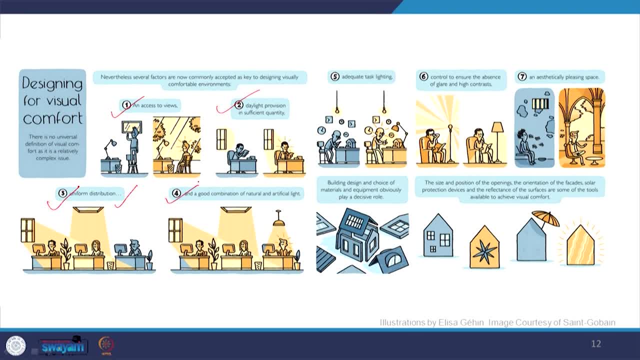 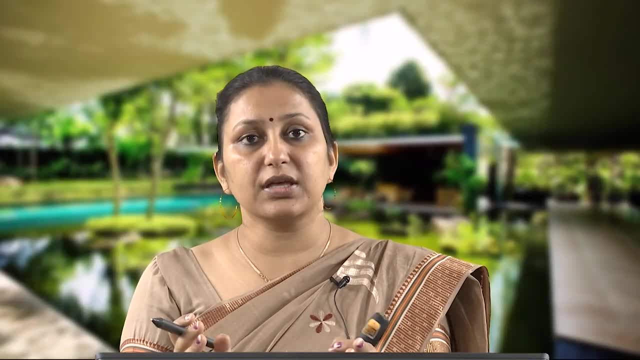 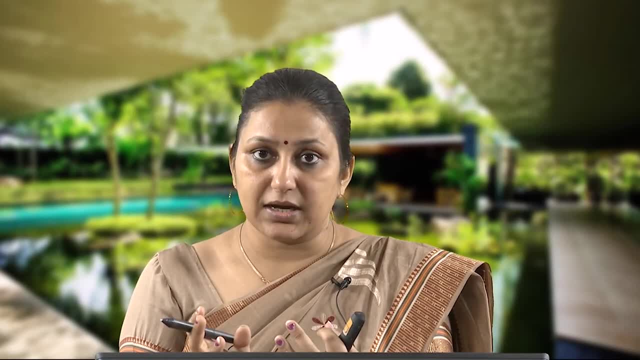 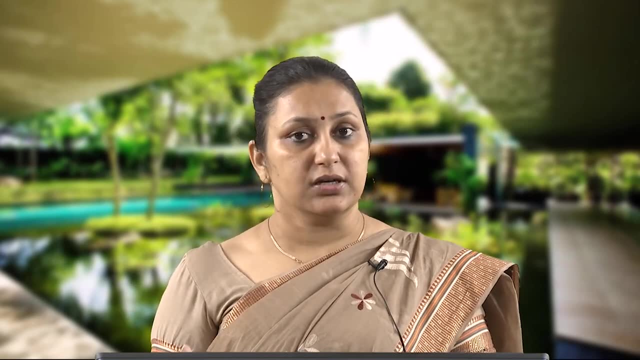 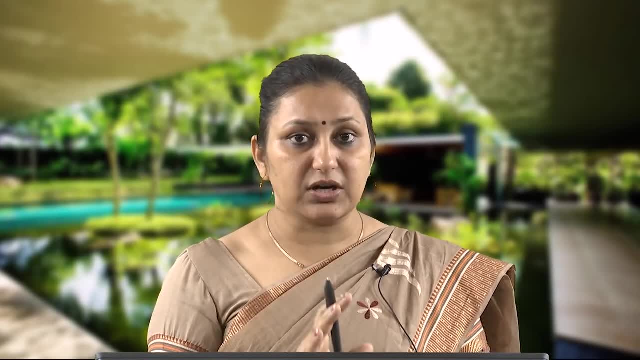 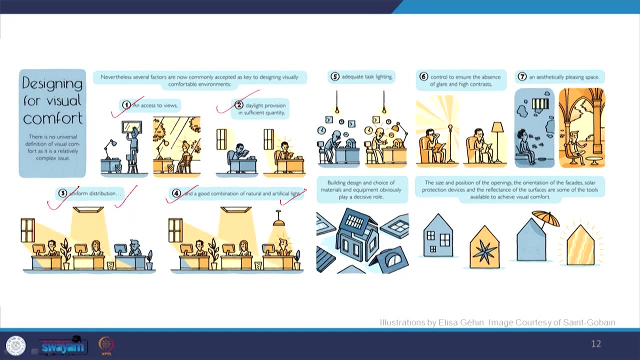 preferably daylight areas, which are which are receiving good amount of diffused light, daylight, daylight combined with provision of artificial light. In addition to that, we should have adequate task lighting, So there may be general lighting in a space and then specific task lighting depending upon an individuals need, which also 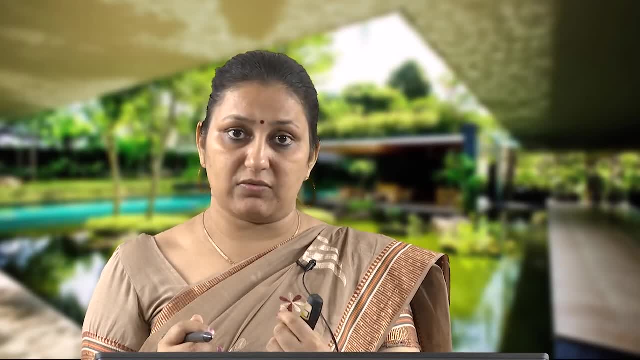 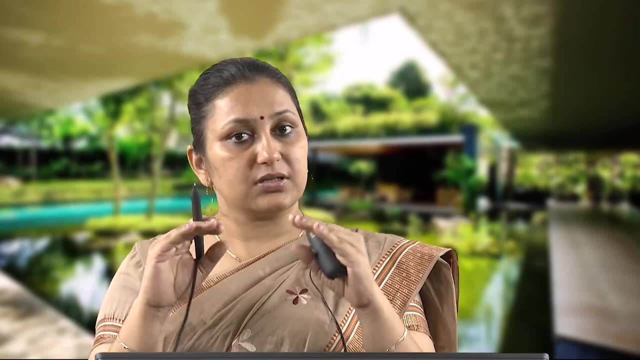 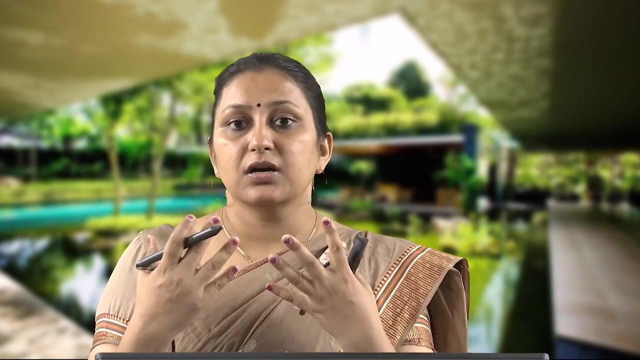 fulfills the need of an individual to control his own environment. Maybe I need more light to work, and there is someone who prefers low levels of light to work, So that personalization of a space giving individual controls is what can be fulfilled through provision of adequate 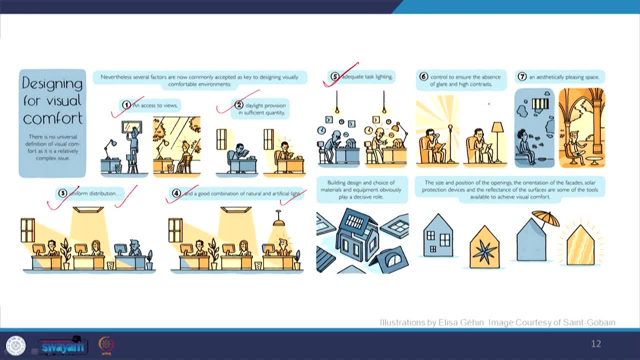 task: lighting. The next is the ability to ensure the absence of glare and high contrast, So we should use such fixtures, such luminaries, where we are able to control the glare. The next is an aesthetically pleasing space. This is a very qualitative aspect, but any 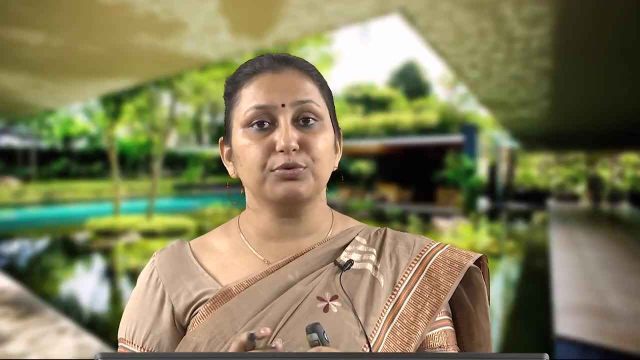 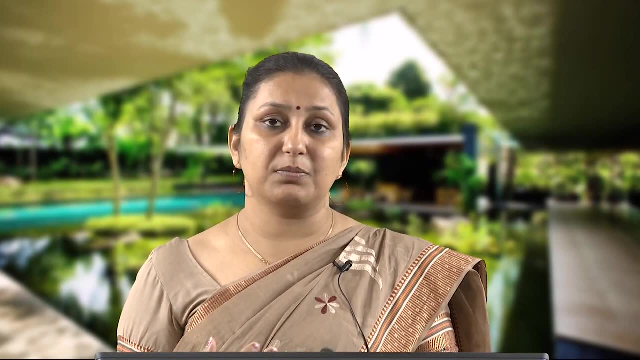 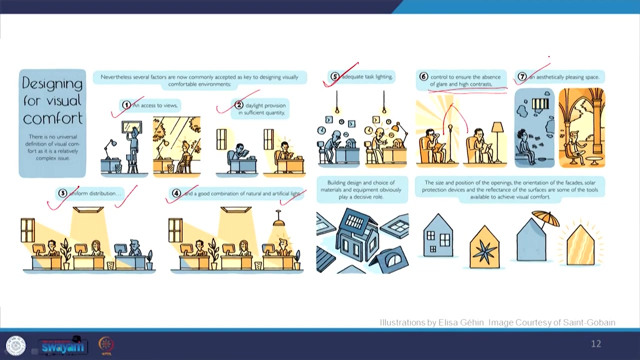 space which is aesthetically pleasing, beautifully designed interiors. These environments enhance the productivity of people. they become, they feel more energetic, they feel more activated to work. So these are few parameters which we can keep while designing any space for visual comfort. 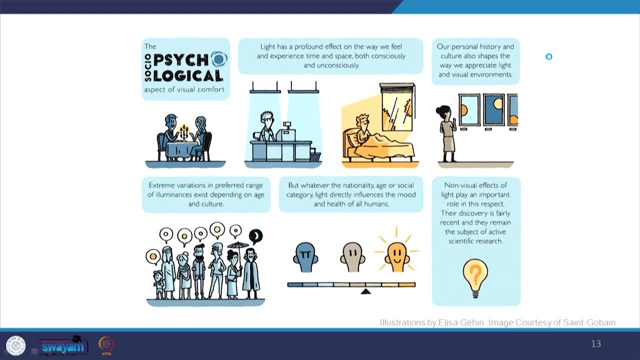 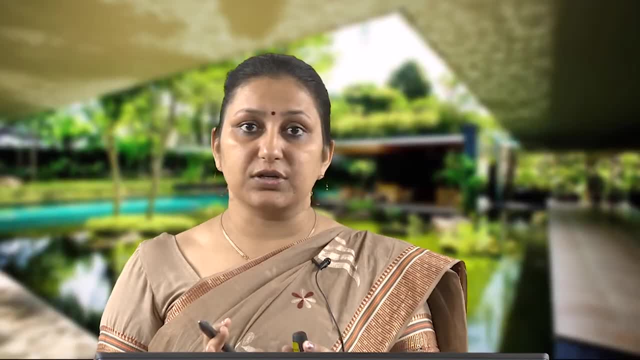 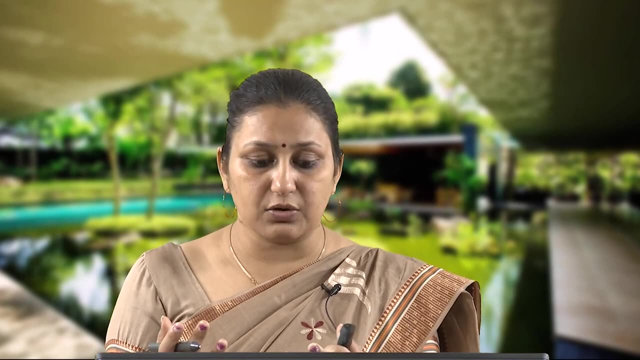 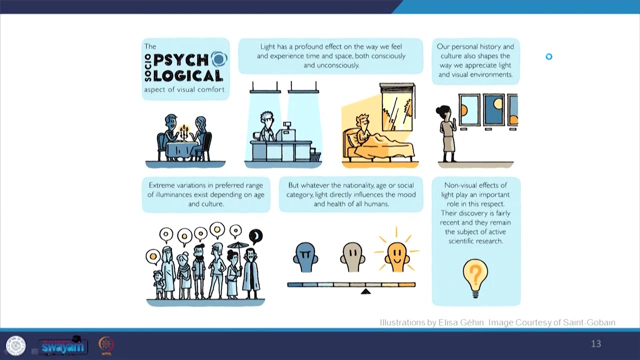 And this is based upon a lot of socio-psychological research where it has been established that good visual comfort, The amount of light, the type of light, quality of light, amount and intensity of it actually has a significant effect on how we feel, how 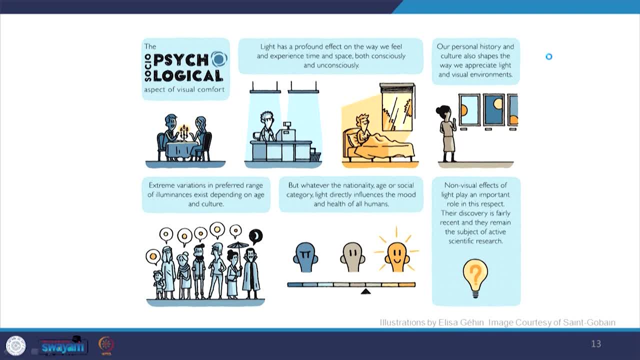 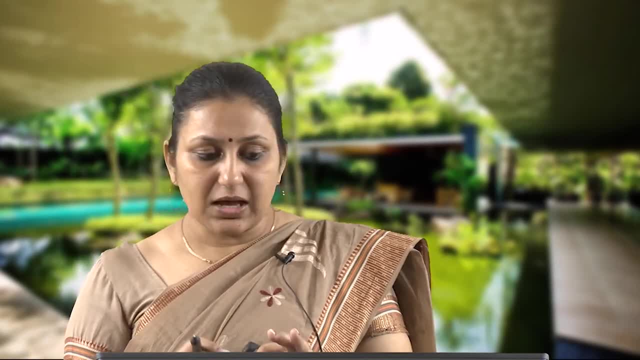 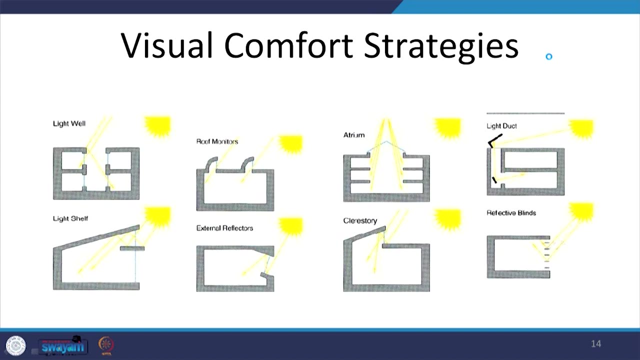 we experience in a space and in time, both consciously and subconsciously. So we have to provide for good visual comfort. Now some of the visual comfort strategies which can be employed to bring in light So we can use light well, we can use roof monitors and atriums where a lot of daylight 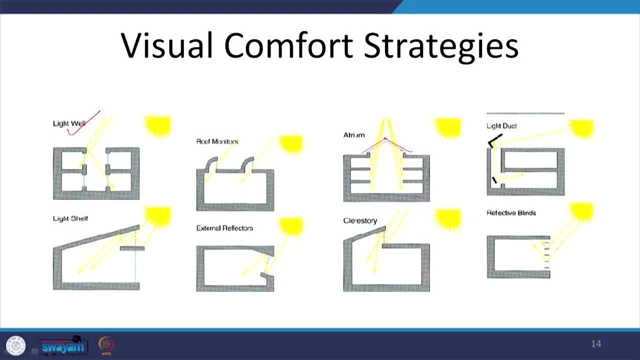 can be brought into the atrium. The courtyards actually serve such purpose. There are light ducts, So this is the reflective side of the material, where the light is actually reflected. It is mirror and if you remember, if you have seen some of the old forts and traditional 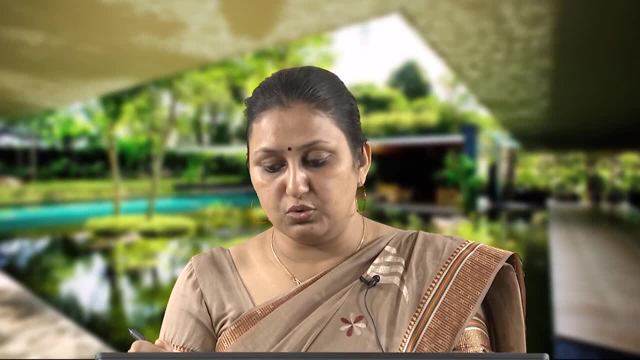 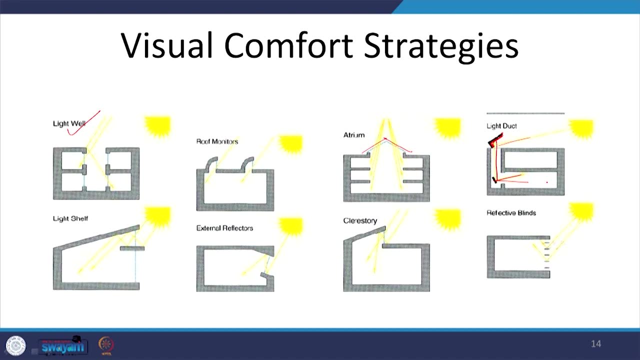 buildings. mirrors were used to bring in light to the deep corridors, to the deep areas inside the buildings. Light shelves we have discussed again this top surface of the light shelf is a reflective surface and it reflects and this light which is received indoors is actually a diffused 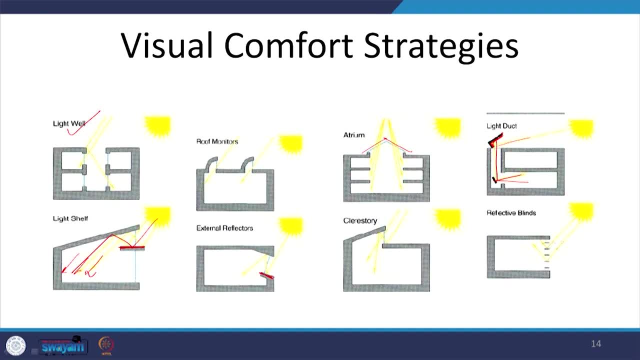 light Similar to light shelf. we have a shelf here, So it is slightly different from this light shelf, but serves the same purpose of reflecting the light and then diffusing it. We have clear story again: reflective surface- here direct as well as diffused penetrates. 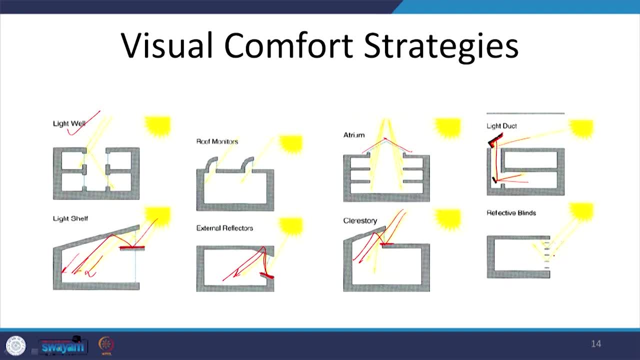 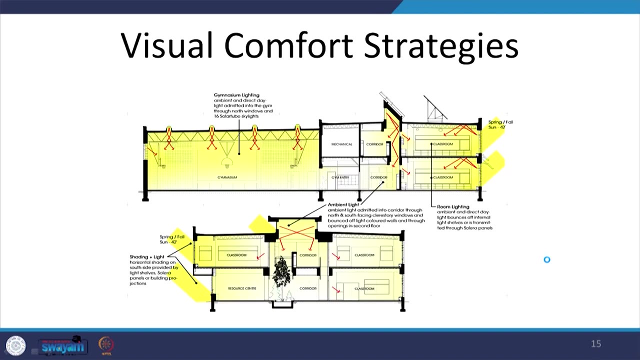 inside, and we have reflective blinds here which are serving Similar purpose as the light shelf, smaller light shelves, as we can see here. Another very interesting strategy which is utilized in case none of these is working is to divide the window in such a manner that a large window, where we have a large window, 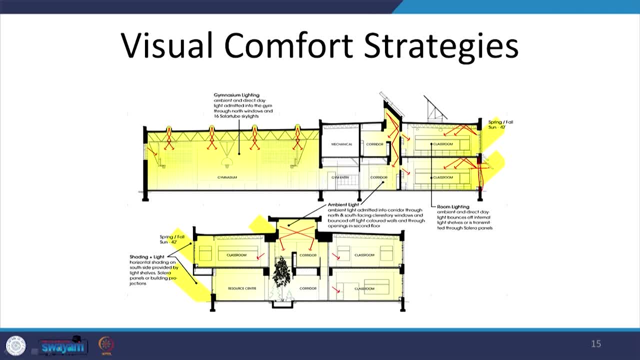 we can divide it. the portion above, the visual part of the window is where the color of the light is reflected, So we can divide it. So this is where the clear glass is used and that part is used to reflect the light, to bring in light and penetrated deeper, while this part of the window will use a tinted. 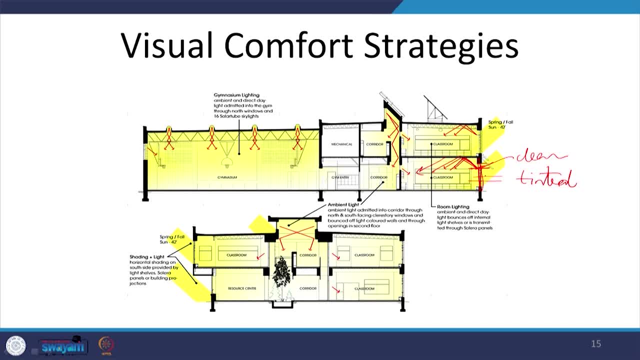 glass Now. this will help in cutting down the glare, So there will be no direct light falling on to the eyes of the occupants- and there is. however, there is sufficient light which is brought in through the clear glass which is above. 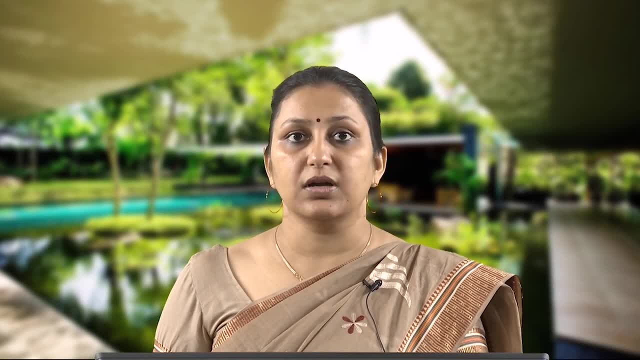 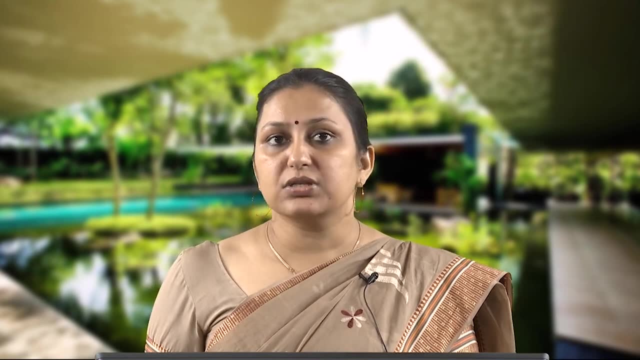 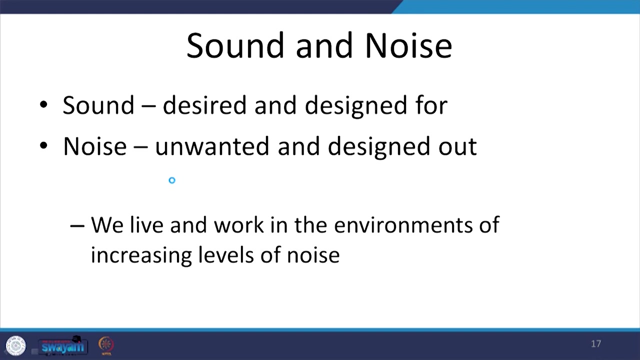 So this helps to bring in diffused daylight into the habitable rooms. Next, we have acoustic comfort. Now, when we are talking about acoustic comfort, we must very clearly understand the difference between sound and noise. So sound is what we have desired and we have designed for, while noise is something which 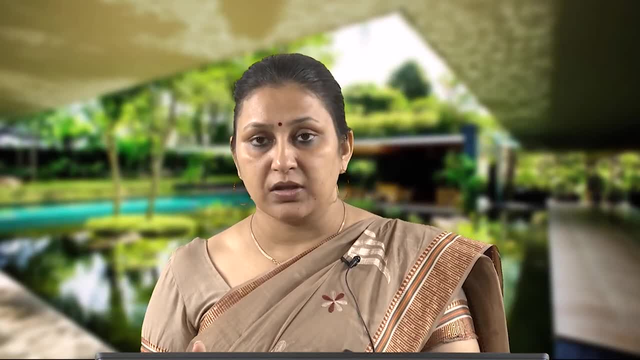 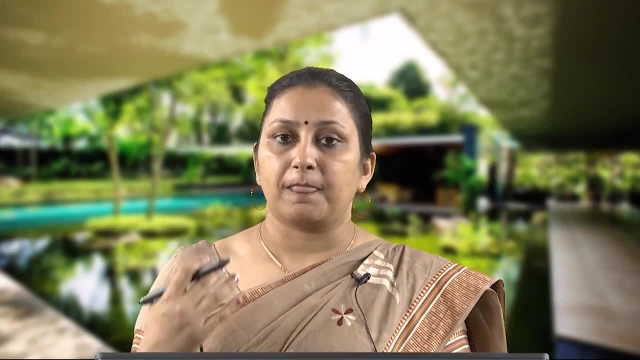 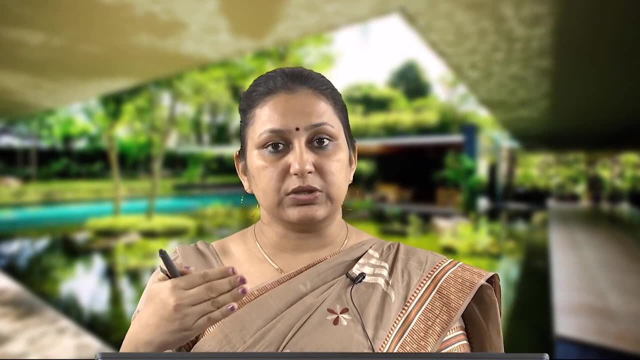 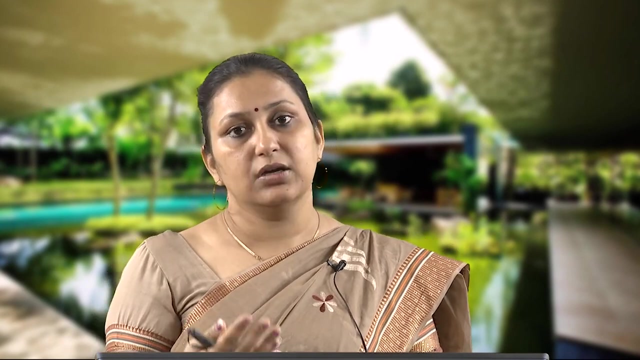 So when, as a teacher, I am in the classroom, what I am saying, the lecture that I am delivering and what my students are able to hear is what the sound is. I should be able to hear what my students have to say. they have to ask and the students 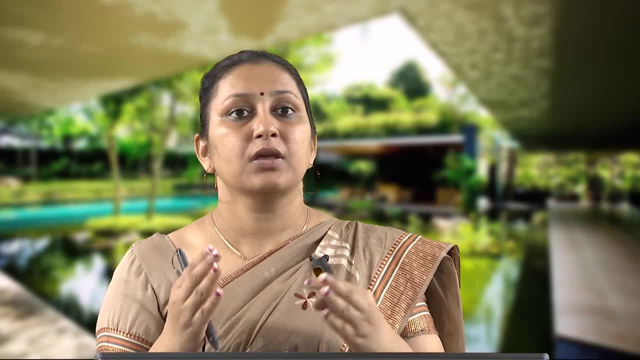 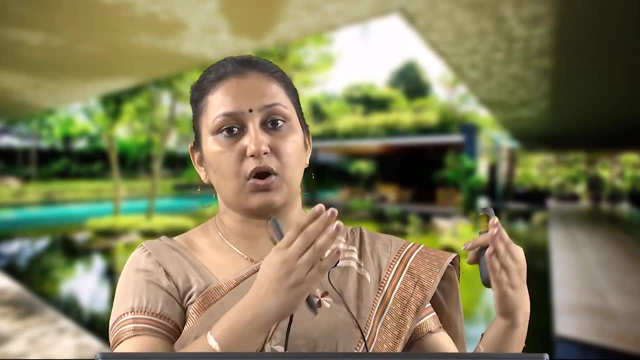 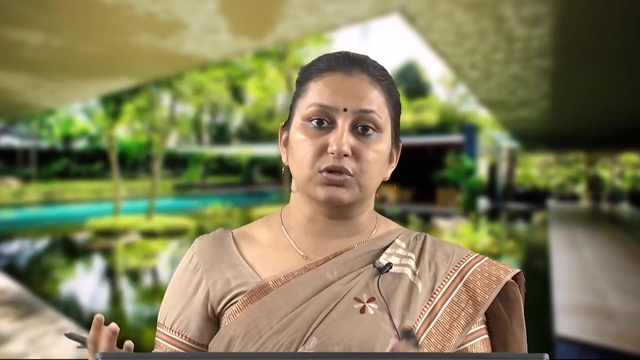 should be able to hear me what I am delivering, While noise is something which is what we do not desire in this space. So, for example, somebody walking in the corridor outside my classroom, a vehicle going by the side of the classroom on the road- so all these noises are unwanted. 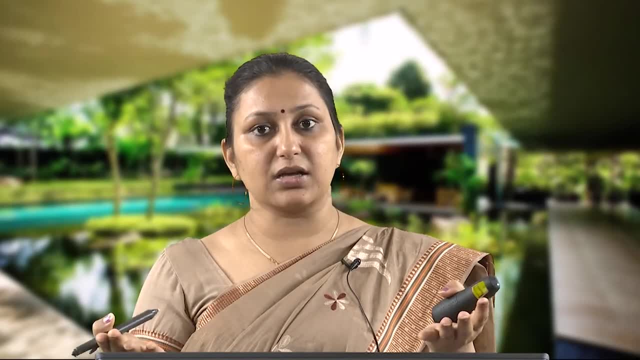 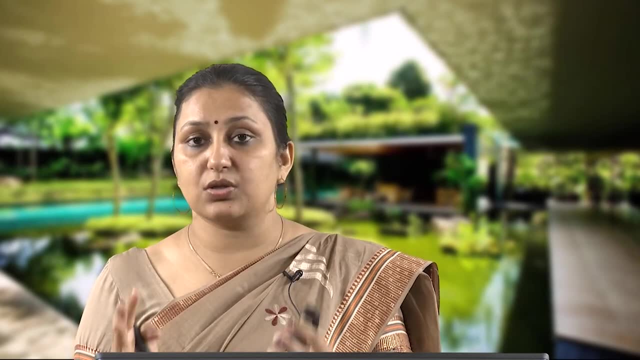 So we want to hear each other clearly while in a classroom, but we do not want any of the noises coming from outdoors to inside of this room. that is noise for me. Now, how do we know how much of the sound is available or should be allowed? 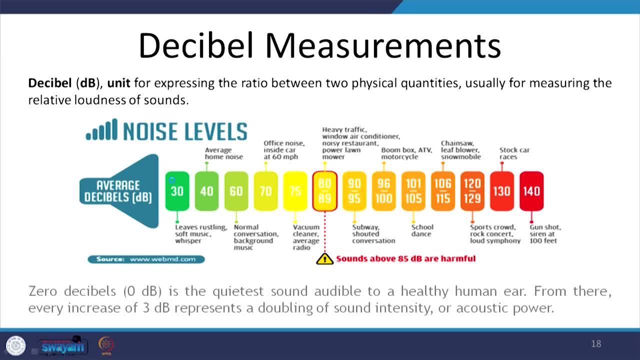 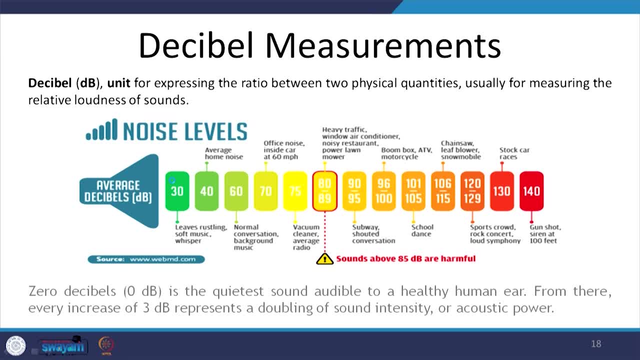 I am sure you have already read the course on acoustics, where you know how we measure. So we measure using decibels. So decibel is the unit for expressing the ratio between the two physical quantities for measuring the relative loudness of sounds. 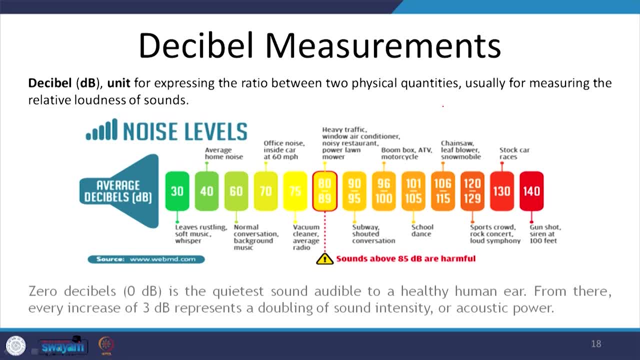 If you look at the average decibels which are required in an office And in a classroom, around 60 decibels is what we would normally require. that is that is what should be maintained. extremely low decibels. spaces which are too quiet are also. 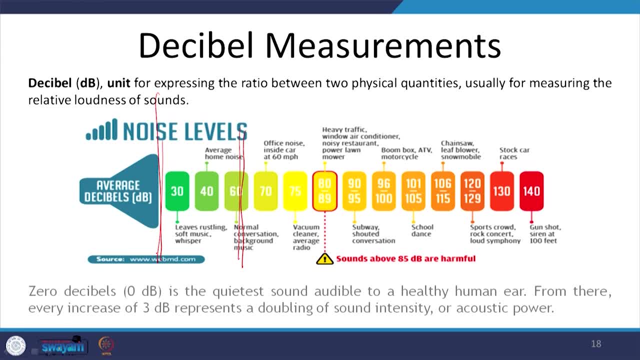 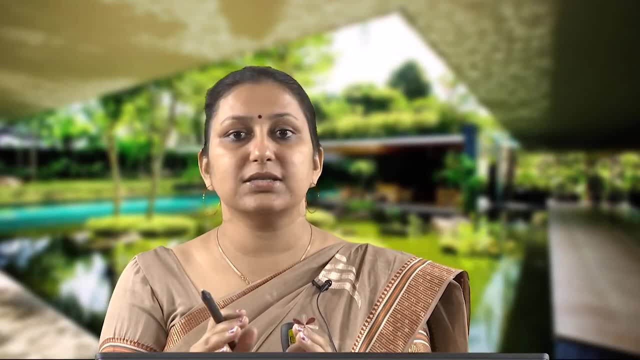 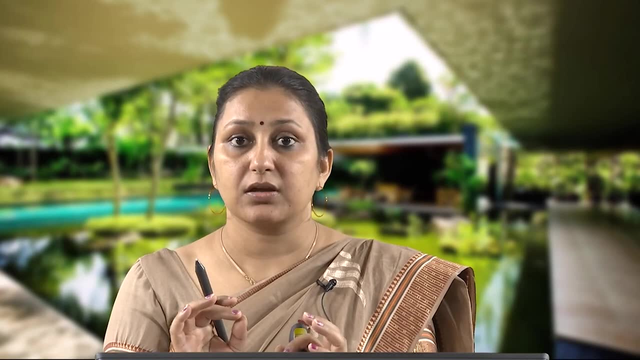 not comfortable. We might be comfortable in those spaces for a very short while. So there was an experiment which was conducted in one of the universities in United States where They were able to bring down the decibels in a space down to 0.. 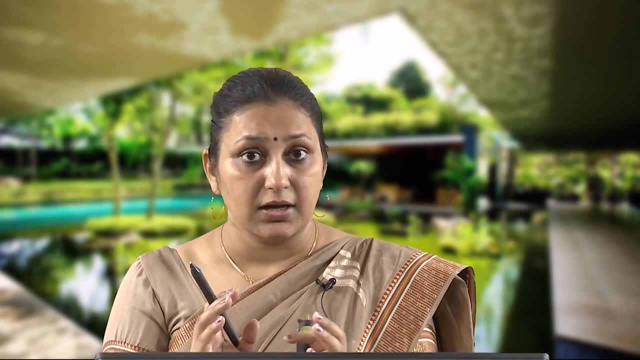 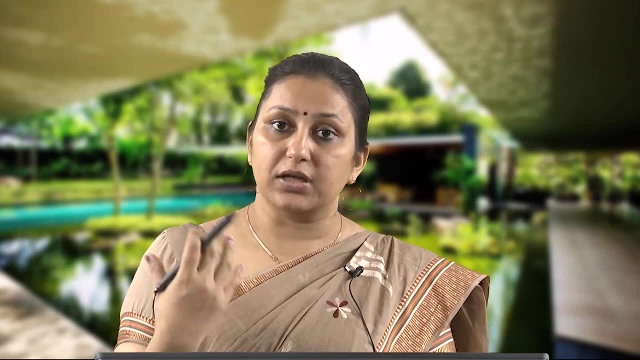 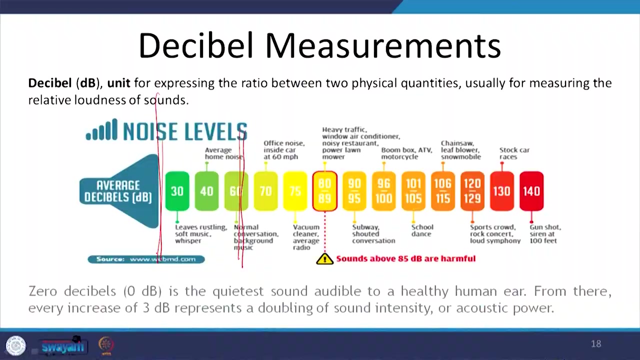 So an absolutely quiet space and at 0 decibels the human beings. we can hear our own blood flowing through our body and it is quite disturbing. So we need a little sound around us which is around 30 decibels is good- 30 decibels. 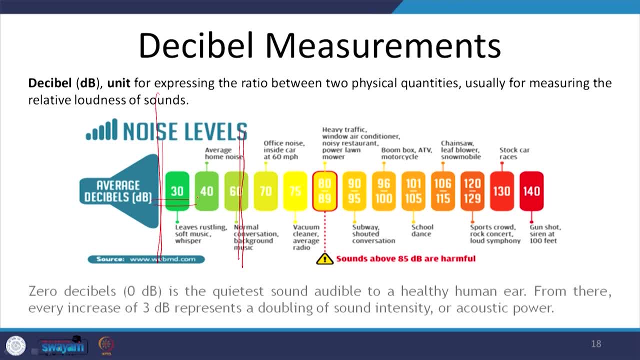 is where you have the leaves rustling, You have the sounds of the nature, Little bit of whisper, and it is quite comfortable. If we look at 40 decibels, this is what we require for sleeping, So around 30 to 40 decibels we can comfortably sleep. 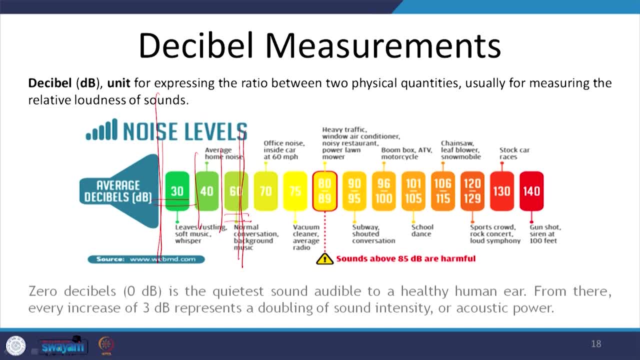 60 is what we would look at, what we want in the classrooms. slightly higher than that is what we would look at. we would be comfortable when we are in an office space where people are moving, People are talking, there are little discussions going on. When we have some average radio being played, little bit of music, vacuum cleaner and all. 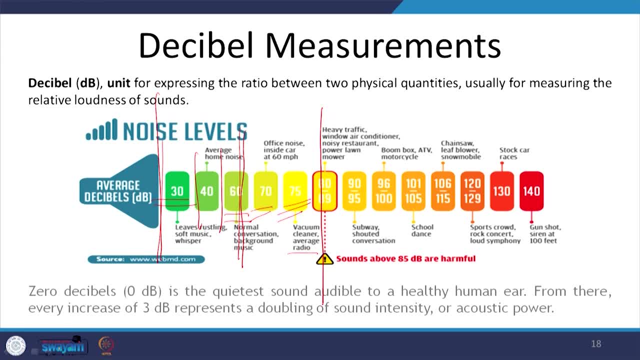 that is around 75 decibels. Now 80-85 is the limit. beyond this it is harmful for the ears. So any sound above 80-85 decibels is noise beneath this, also depending upon the space it is. 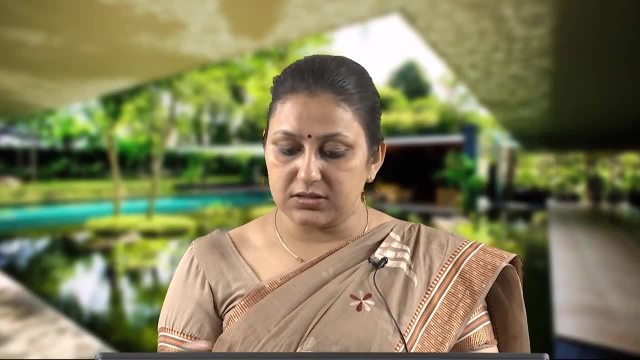 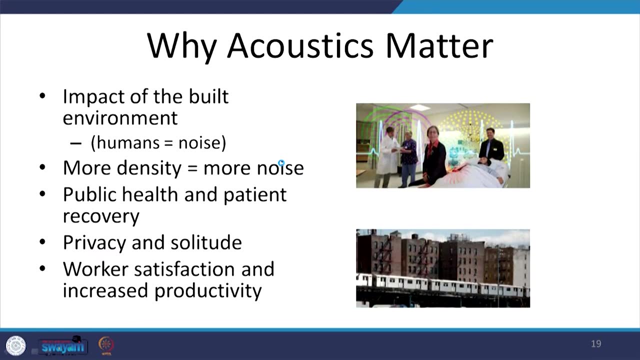 So it has to be qualifying as noise. above this, it is definitely harmful and noise So, depending upon the quietness that you require or the amount of sound that you require, the space has to be designed. It will impact the health of the occupants. the amount of sound which is present: amount. 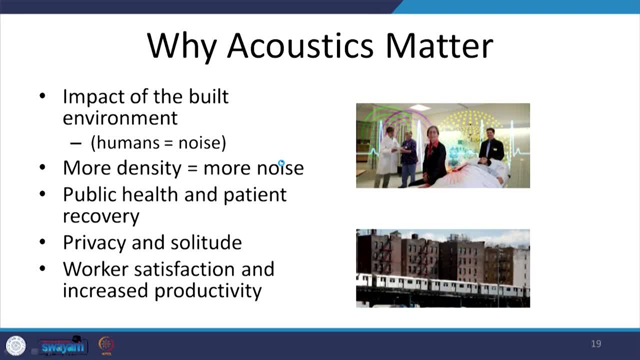 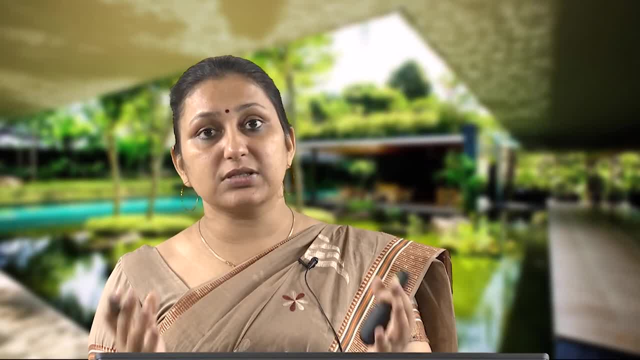 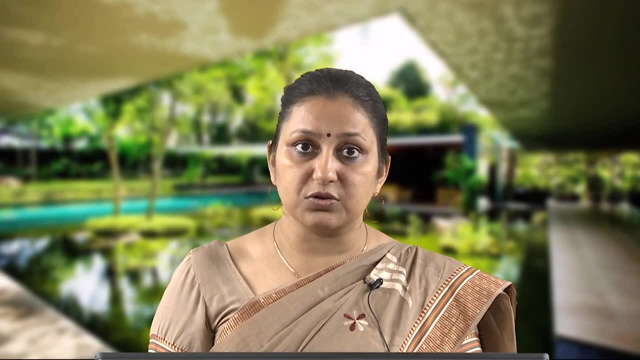 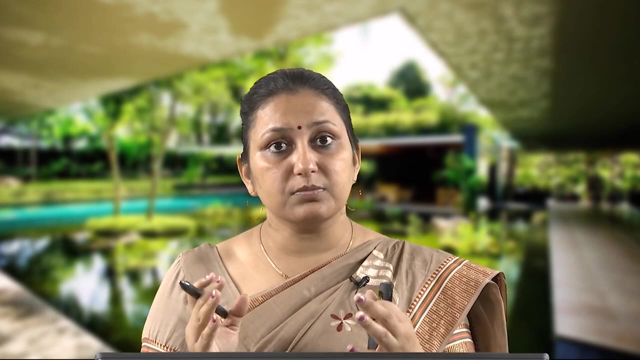 of noise which is present Focus upon varying levels of privacy. So in areas which are more private, suppose I want to have a private discussion in a conference room even when I am in an office. such areas would require more acoustic treatment, For example the theaters. they require more sound acoustic treatment to provide for the 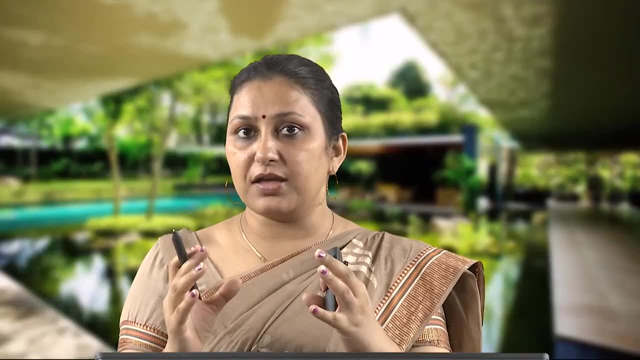 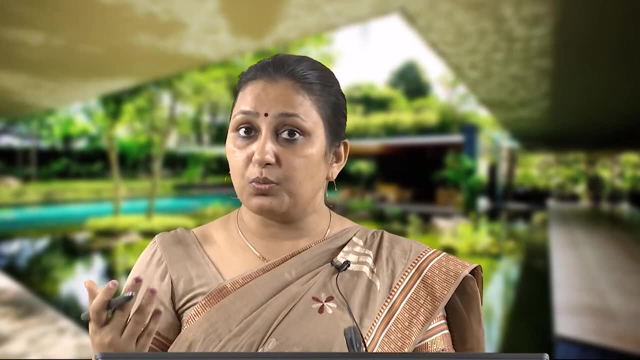 So when we have a reverberation or time of 3.5, because there are different types, different intensities, different notes, different musical waves, The musical waves which are hitting our ears, that is where the musical sound will sound. 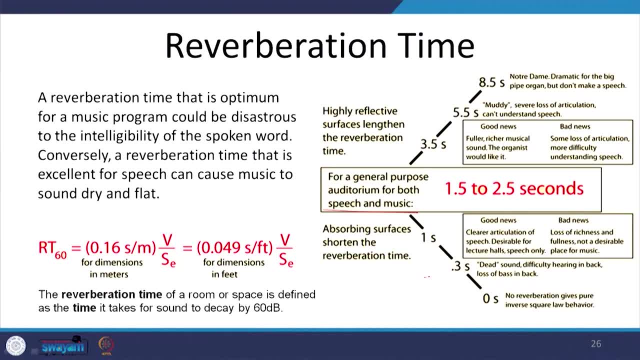 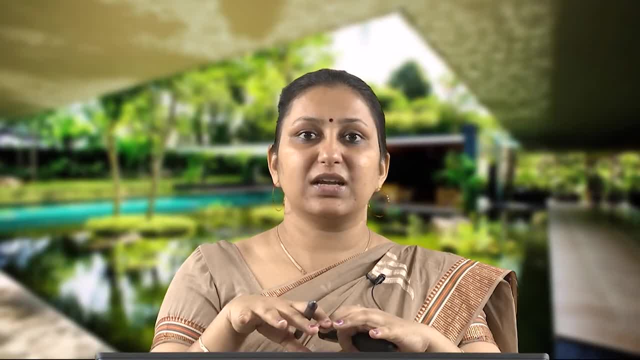 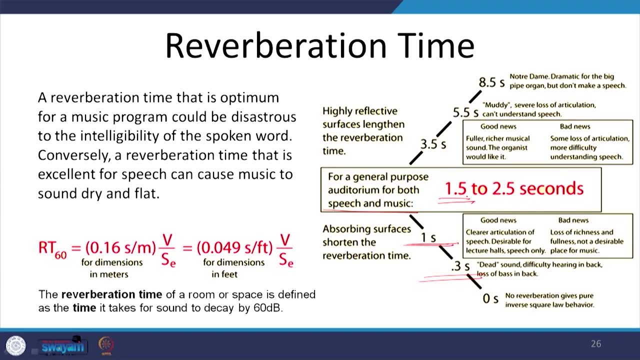 fuller richer. If we have less reverberation time, less than 1, it will be perceived as a very dead space. it will be perceived as a very dead sound, while it may be good for speech. So around 1.5 second of reverberation is good for speech. 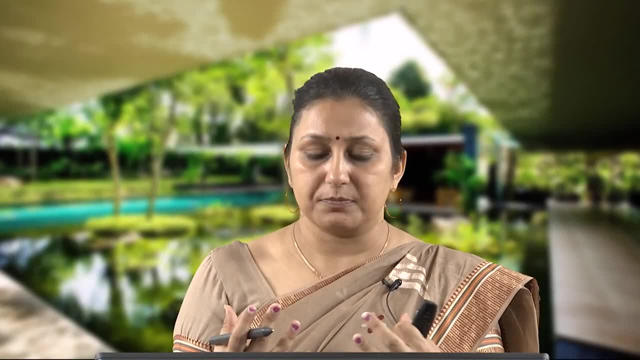 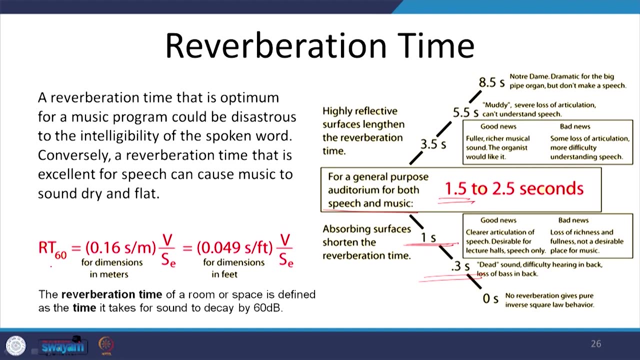 So little bit of hard surfaces should also be there. that is when it sounds good. Now that is this. reverberation time is calculated on the basis of the total surface area, equivalent surface area, which takes into account the absorptivity, the absorption coefficient of 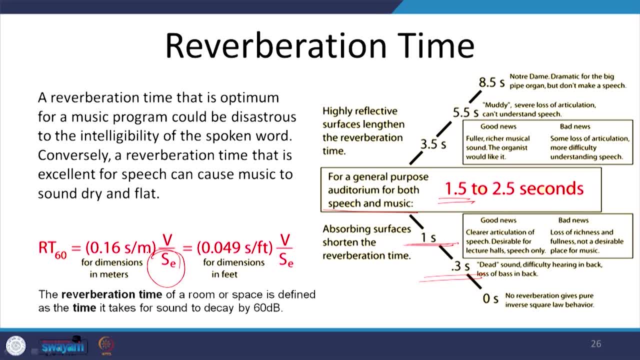 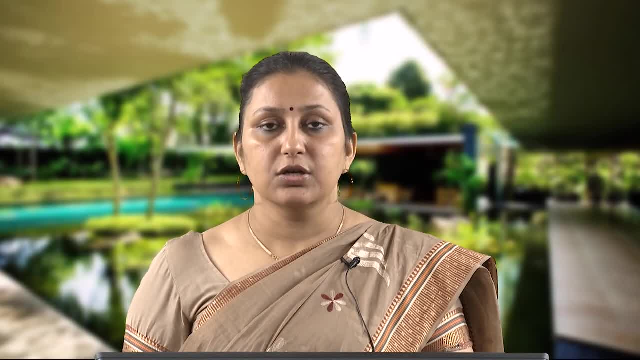 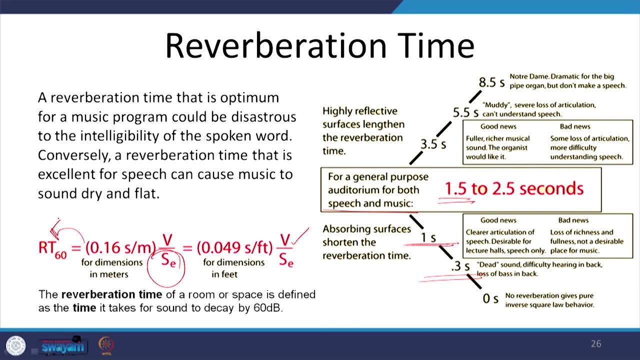 the surface and the surface area, all the different surfaces and their absorption coefficients put together, and also the volume of the space. So together these two result in a reverberation time designing for auditoriums, theaters. reverberation time becomes very important, but often we 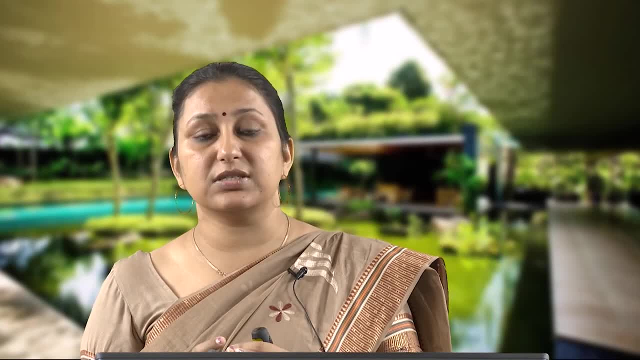 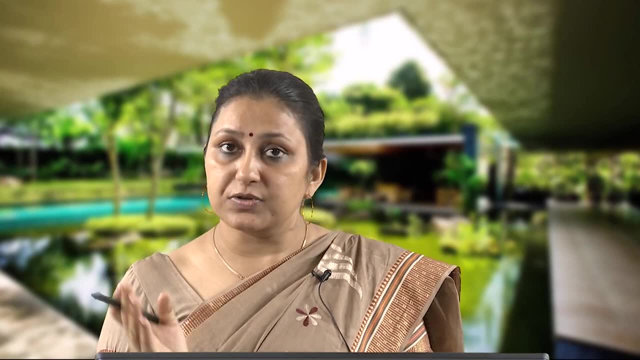 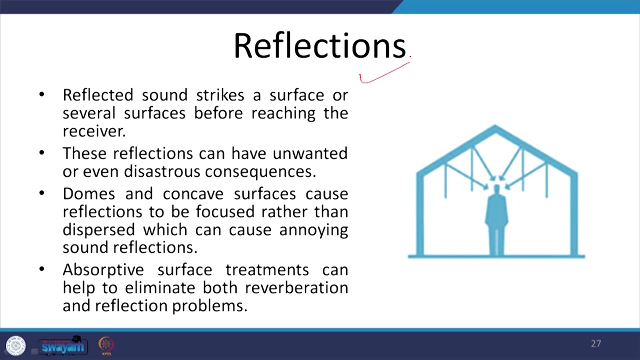 forget about it when we are designing classrooms, when we designing offices. but we should take into account, take care of the kind of surfaces which are being used. Here we are also talking about reflections. the reflection results in reverberation. So how the sound is going to be reflected, so it depends upon the material as well as 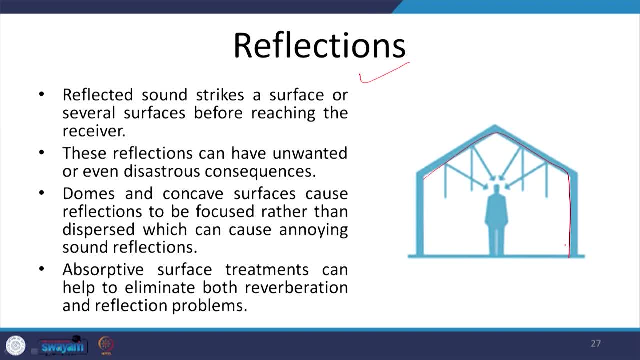 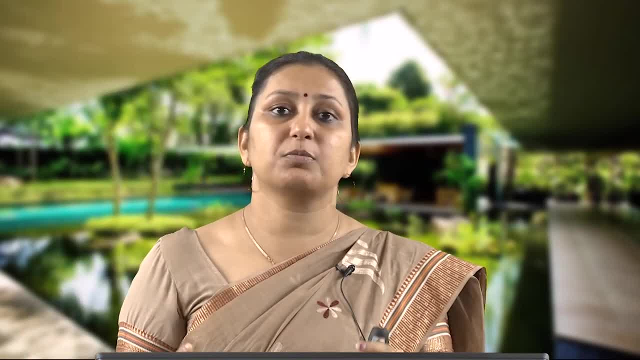 design, So how the sound is going to be reflected, how many times will it be reflected, will result in reverberation. So for any good classroom or office a reverberation time of around 1.5 is a good reverberation. 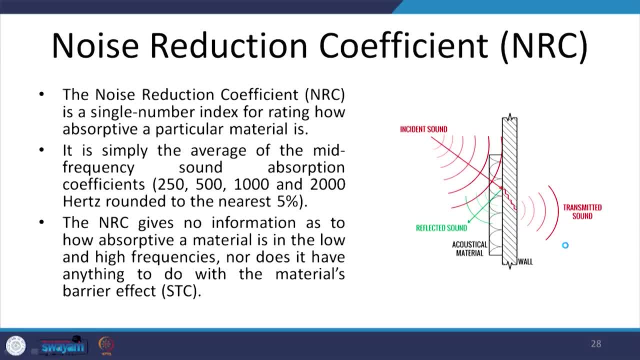 time and we should choose materials effectively. Here we are also talking about noise reduction coefficient. This is an. this is a measure of the material, individual material, where we know how much of the sound can be absorbed by the material. So an higher number of noise reduction coefficient implies that larger is the amount which can. 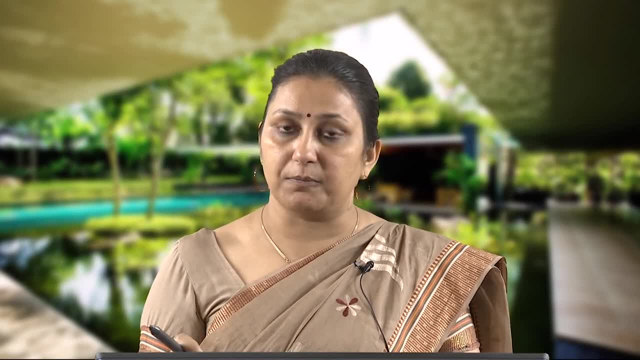 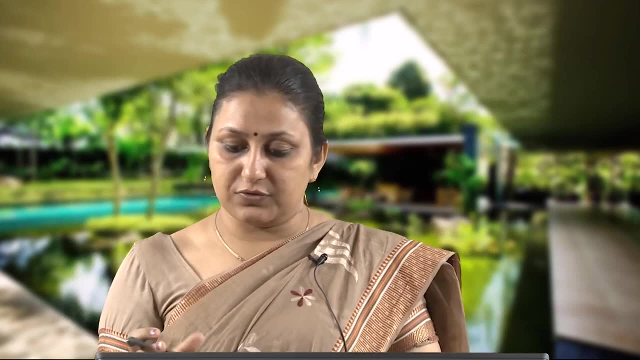 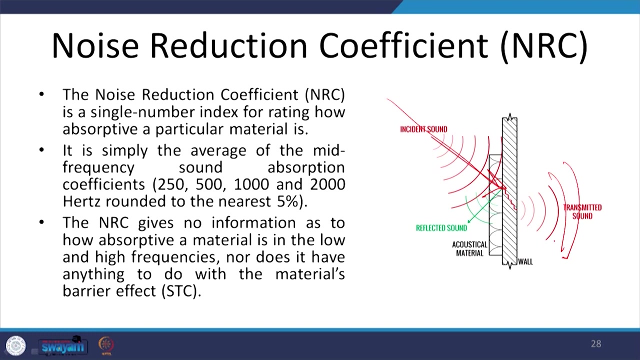 be absorbed or diffused by the material. lower is that number, lower is the amount of sound which can be reduced. the reduction of the sound, So of the incident sound which is there, how much is transmitted to the other side, is the measure of NRC noise reduction coefficient. 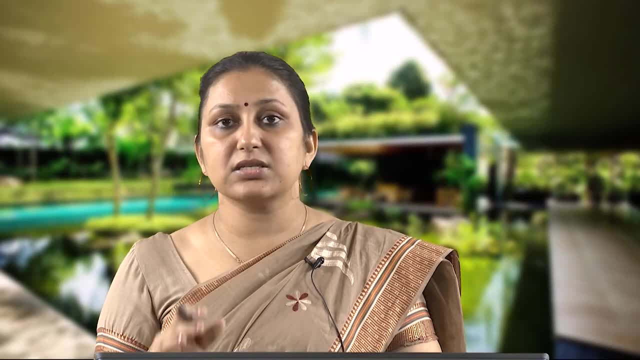 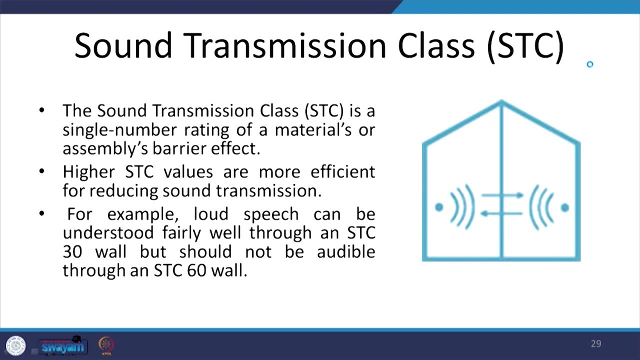 Lower is that number, the better is this material for sound insulation. The same is further taken to understand or classify the materials in different classes. there is sound transmission class STC. So higher the STC values are, the more efficient is the material for reducing sound transmission. So it is an inverse of NRC in a way. 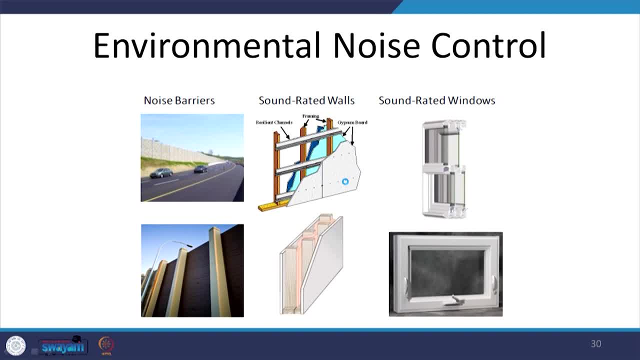 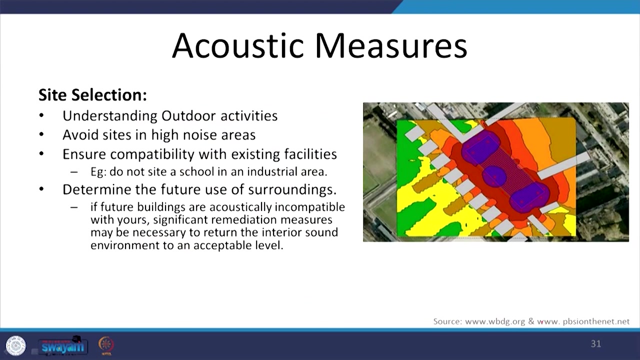 Once we understand what these materials are and what are requirements from design is, we can look at the different strategies for sound barriers. we can use the sound rated walls, which are STC, and we can look at these windows, which are also sound rated windows. There are design measures which we can use, for example, the selection of site. So understanding 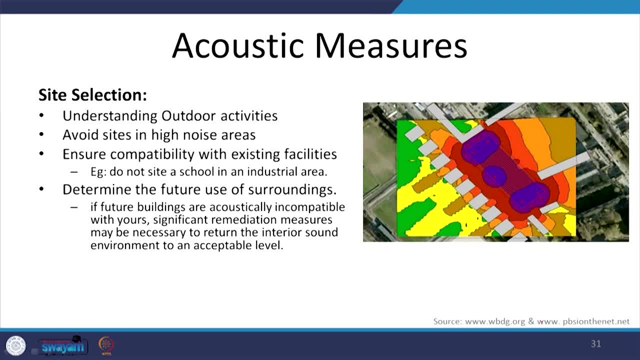 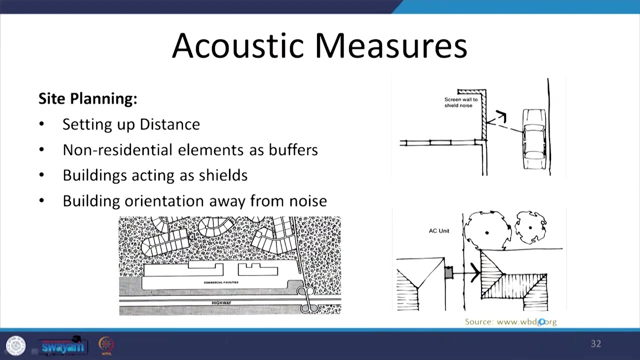 from where the sound comes to a site. So we can do in such a manner that noisy activities, which can be performed with high noise amount, are placed in the high noise areas and the quieter activities are placed in the quieter areas. We can look at the distance of the site, we can look at different elements. 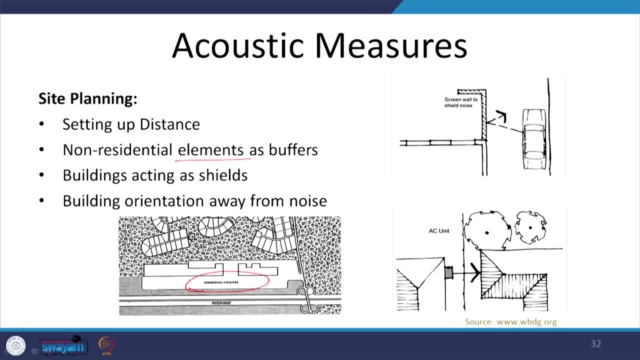 non residential elements, for example commercial facilities. So this is a highway going and this is the residential. So between the highway and the residential area a huge commercial facility has been developed where it acts as a barrier of sound to the residential area. So this is building acting. 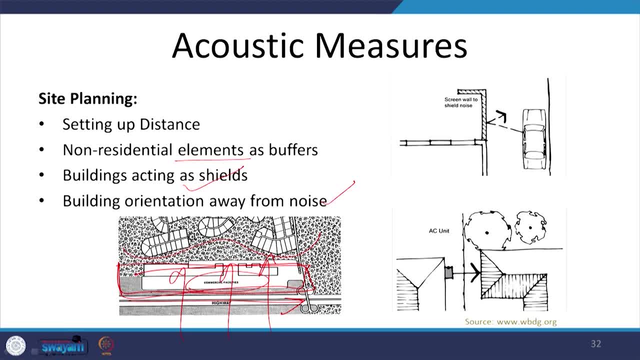 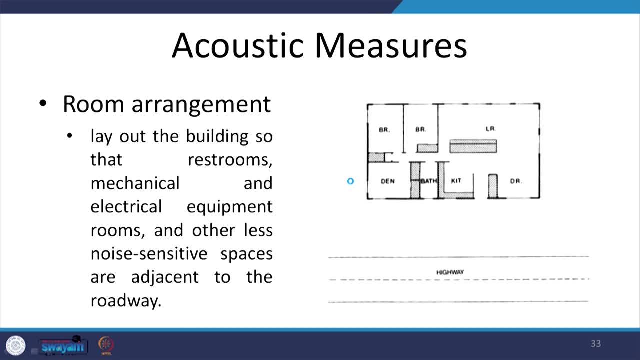 as shields and also orienting the building away from the noise, So we can orient the building in such a manner that the noise is cut away. We can also look at the internal arrangements Now. bedrooms are the quieter areas where people sleep during night, So they can be. 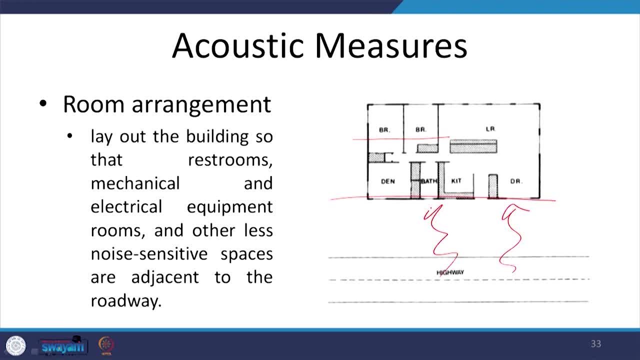 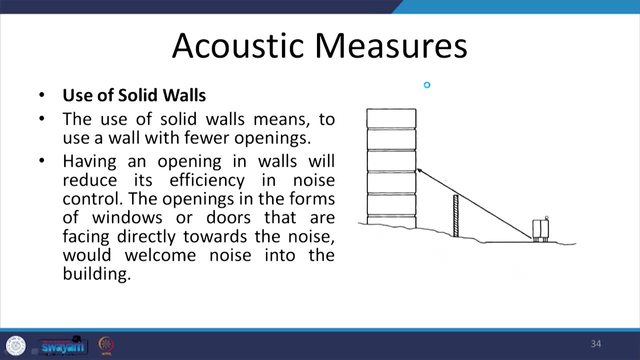 kept away from the noise, creating site noise, the source of the noise. So more active areas, for example the drawing rooms and kitchens and bath areas, they can be used as a buffer, as an acoustic buffer, and the bedrooms can be at towards the quieter side. 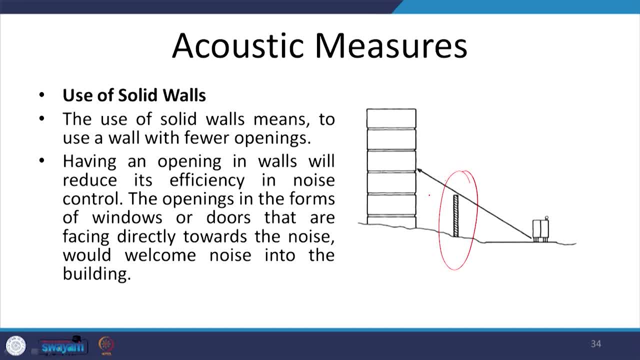 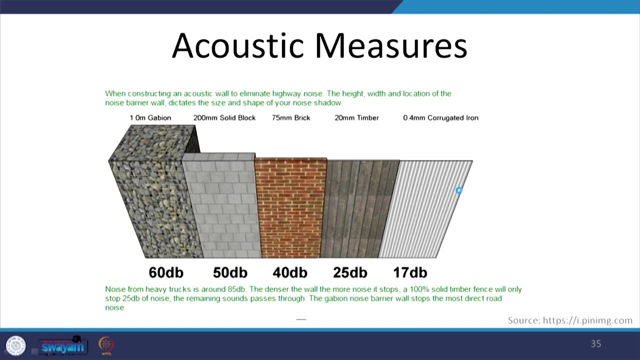 There are multiple other measures, For example, using walls, solid walls, as acoustic measure. So this is a highway going and this actually acts as an acoustic measure. Besides walls, trees can also act as acoustic measure. If we are looking at materials, we should understand the difference between each material. 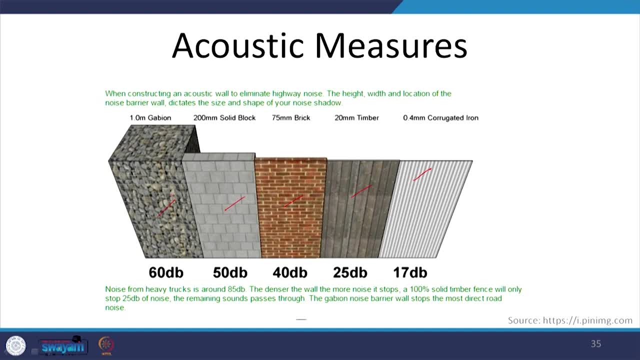 and the amount of sound reduction insulation that each of these materials provide. So the walls, the regular walls, provide around 40 decibel of sound insulation difference from the source to the sink side. If you want around 60 decibel around 1 meter of gabion is a useful strategy, a useful material. 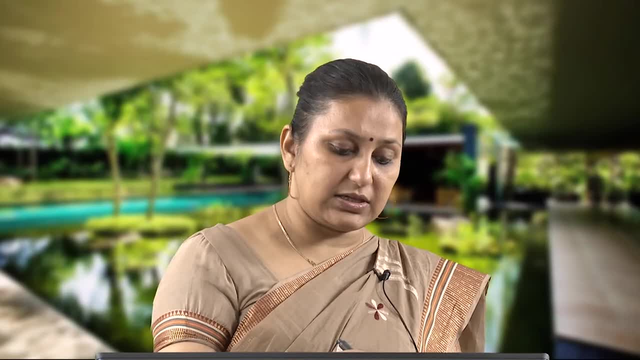 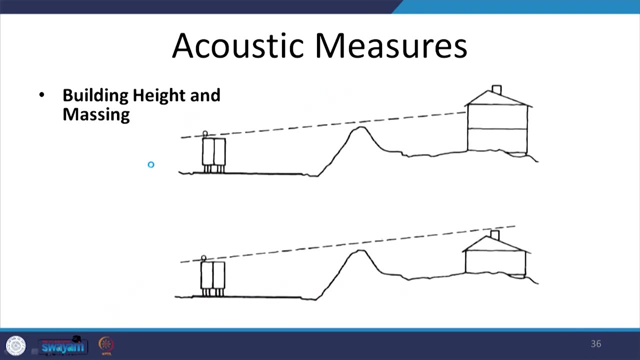 but it is a very thick wall and we should also see that it is porous and that is what causes a lot of sound reduction to happen. There are other design measures, for example adjusting the building height depending upon the topography and the site features, which are available. 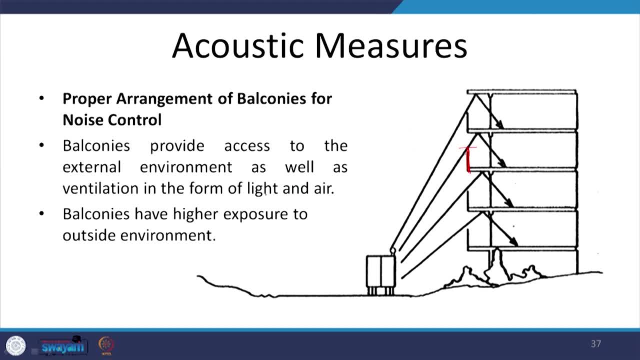 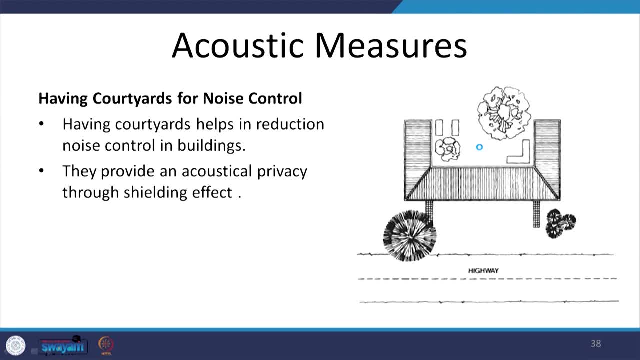 For example, designing the balconies in such a way that no direct noise is hitting into the space. it is coming into the space. Having courtyards for noise control. So, for example, in this building the courtyard is facing away from the highway and this side. 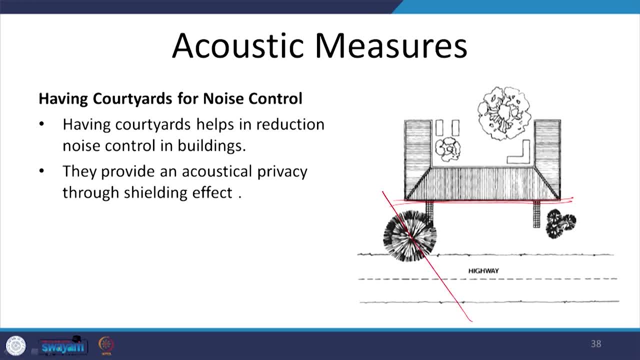 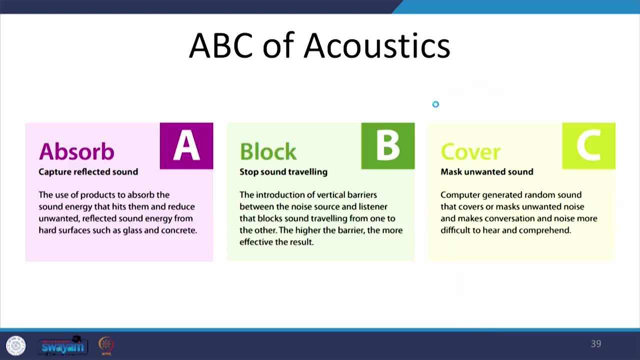 would be a blocked side. So the sound, because it is, travels straight, So there will be less of sound which will be available in this courtyard. To conclude it all we can say, there are three fundamental ways in which acoustics of a place. 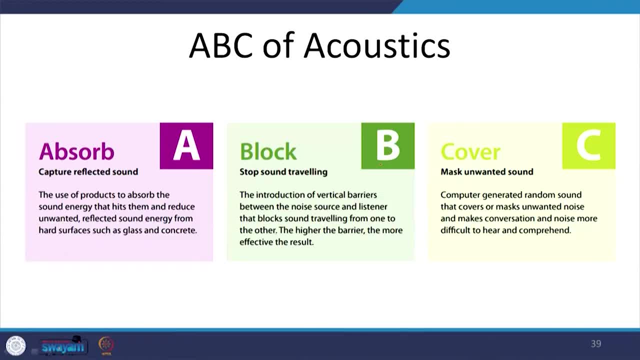 of a space can be designed that is A, B, C, Absorb, Block and Cover. So first is acoustic insulation. Second is to capture the reflected sound by using appropriate material, absorptive material. Second is to block the sound from traveling by introducing the vertical barriers, the 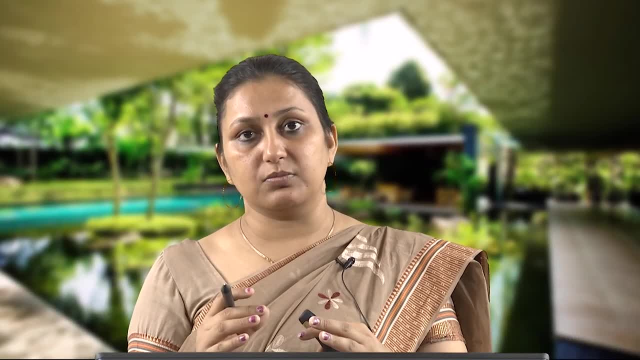 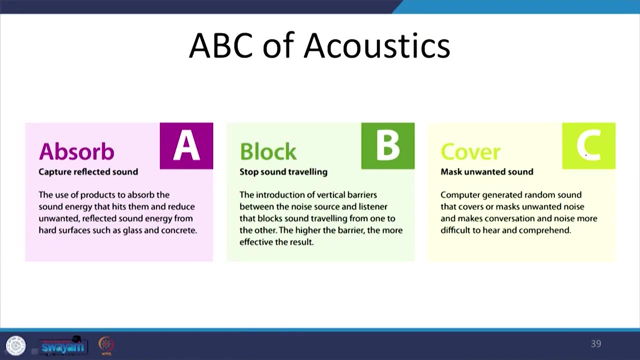 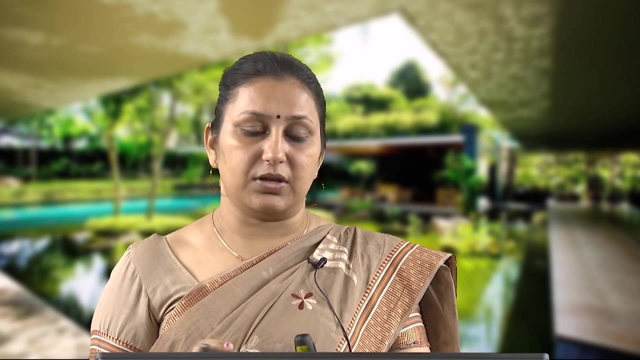 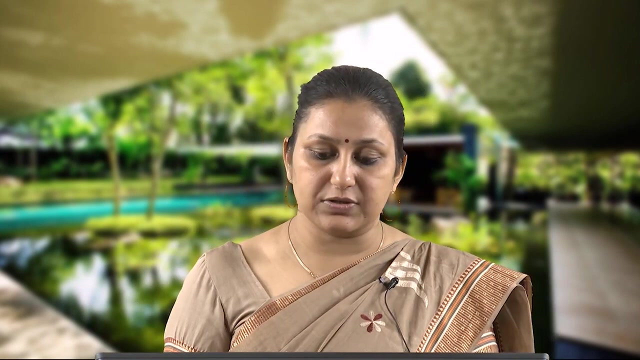 barriers to this sound which can be possibly disturbing. And the third is to cover the unwanted sound, to mask that sound by providing certain covers. So which is what we see in our buildings happening Very quickly, going over the kind of problems that we have we often see in our offices, and 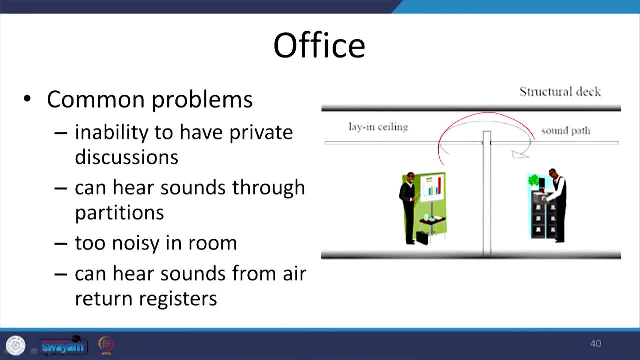 our classrooms is: we have a lot of noise traveling through the ceiling, through the ducted area. There is inability to have private discussions- and we can. the partitions are so thin that we can hear through the partitions and there is no privacy and it also becomes noisy. 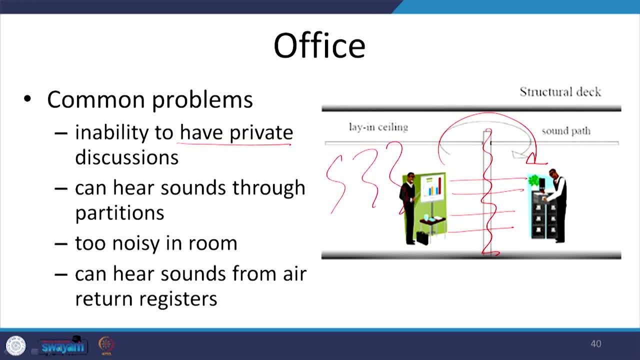 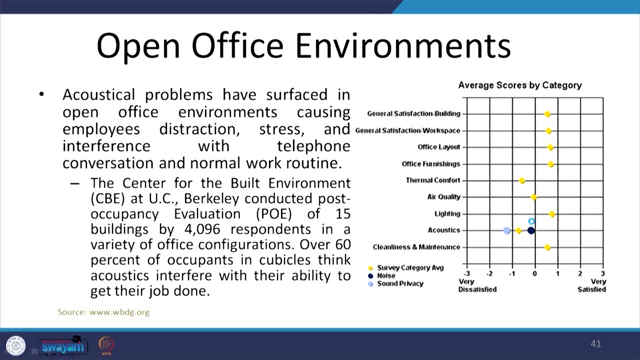 is a lot of noise happening in this area. the area which is supposed to be quiet also receives a lot of noise. So these are some common problems which are there in the office environments and there was a research conducted by Center for Built Environment at UC Berkeley and there people 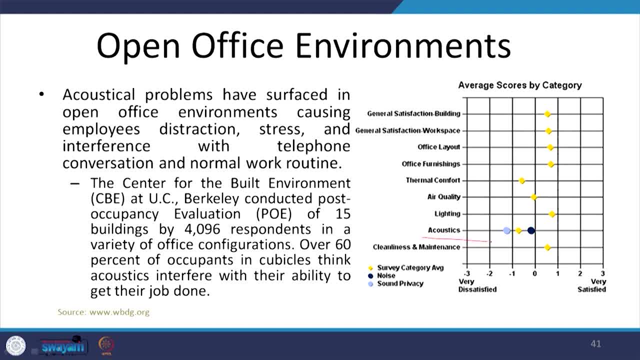 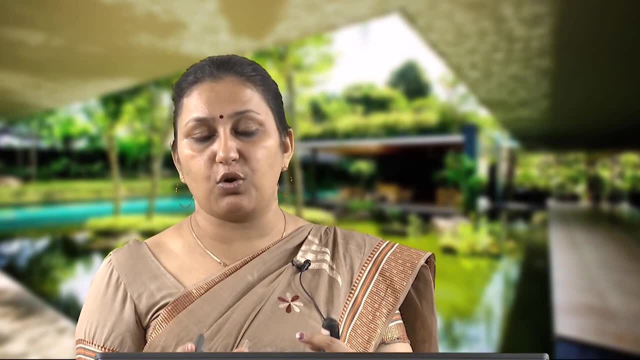 felt dissatisfied, uncomfortable, only because the acoustics was not good For everything else they were quite comfortable, satisfied, but because of acoustics, because this was so noisy in an open plan office. So this research was largely on open plan office environments and people felt dissatisfied. 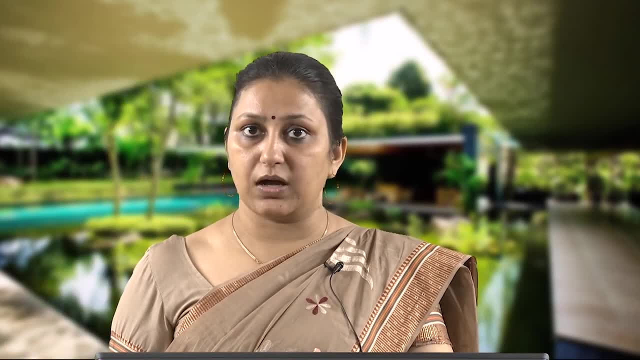 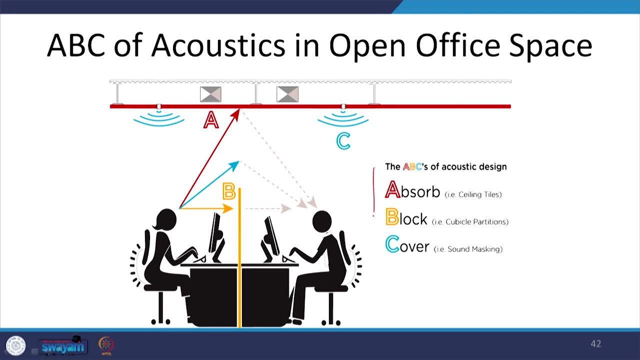 simply because the acoustics was not comfortable. So when we are looking at strategies in an open office space, we are again looking at the ABC. We are looking at the ceiling, The ceiling material, which is reflect, which is absorptive, we are looking at the partitions. 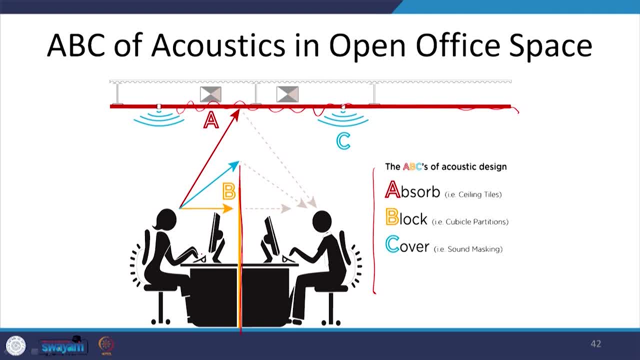 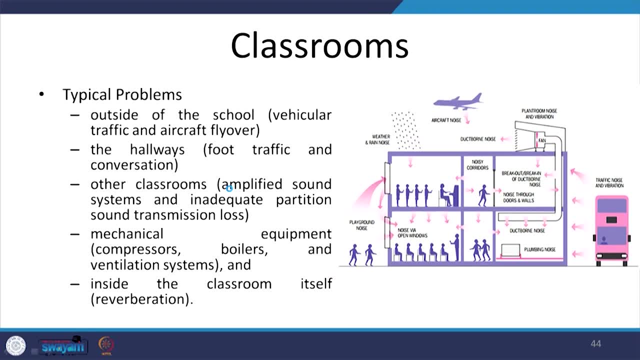 which block. We are looking at the masking of the sound through provisions of absorptive material here. Similarly, we have problems for classrooms where there is outside sound, maybe the noise of traffic or the noise of children playing in the playground inside the room.